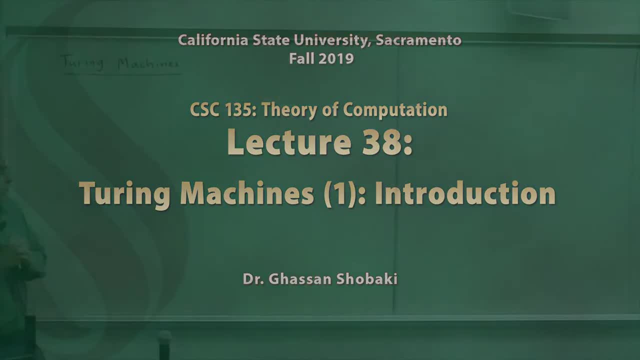 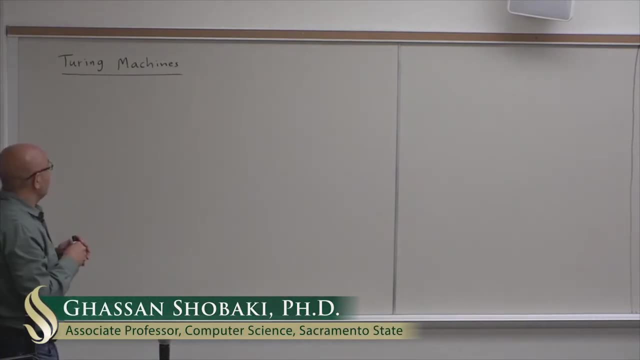 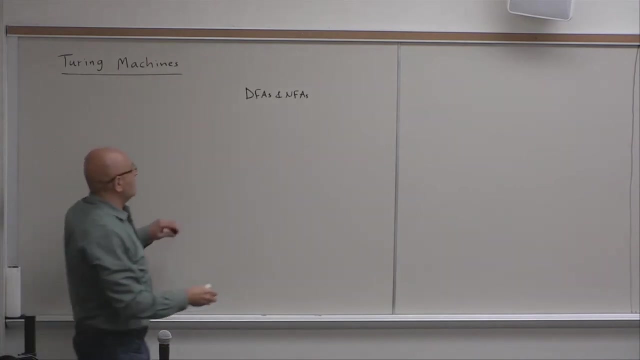 So today we will be talking about Turing machines. So in the previous lectures, you know, we talked about DFAs and NFAs for recognizing regular languages, And we talked about non-deterministic push-down automata for recognizing context-free languages. Now, today we will introduce an 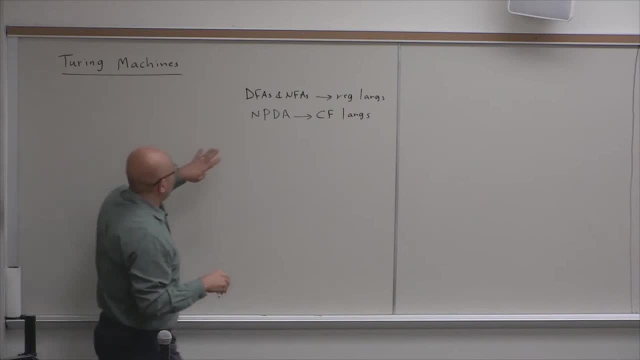 even more powerful machine that recognizes a larger set of languages. In fact, you know, as we will see later, the Turing machine can do anything that a general-purpose computer can do. So, as we will see, a Turing machine can be a theoretical. 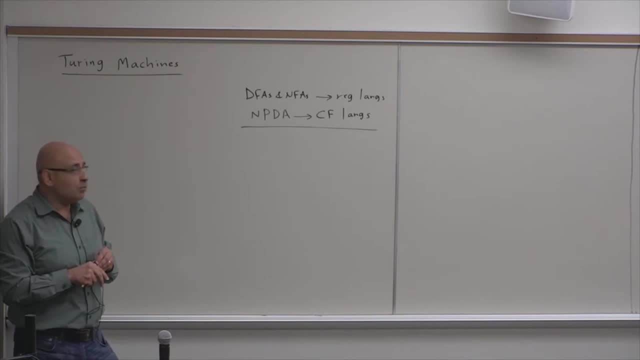 model for a general-purpose computer. It can do anything that a computer can do, Or in fact, it's used as a formal definition of an algorithm. So an algorithm is a well-defined sequence of steps for solving a problem, So anything that you can solve using computers. 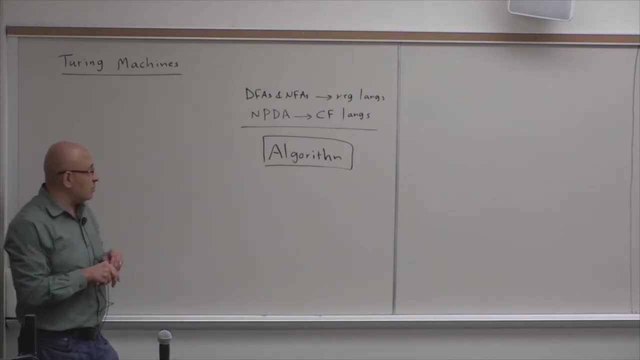 you can do that with an algorithm, Any solution that you, any program that you write, this program implements an algorithm And that algorithm is just a sequence of steps for solving a problem And, as we will see later, we will be talking about Turing machines. So today we will introduce an even more powerful machine that recognizes non-deterministic push-down automata for recognizing context-free languages. In fact, you know, as we will see later, the Turing machine can do anything that a general-purpose computer can do, Or in fact: it's used as a formal definition of an algorithm. So, as we will see later, the Turing machine can do anything that a general-purpose computer can do. And, as we will see later, the Turing machine can do anything that a general-purpose computer can do, Or, in fact, it's used as: a formal definition of an algorithm Array-weekly. there are some Lös, though, that we have done and from our stand-Right, which is to say the rule of the 얠, ricochetslax, steppingrr, ras, which will be very useful in어� nunca maltrés yok, It's also very important to notice. 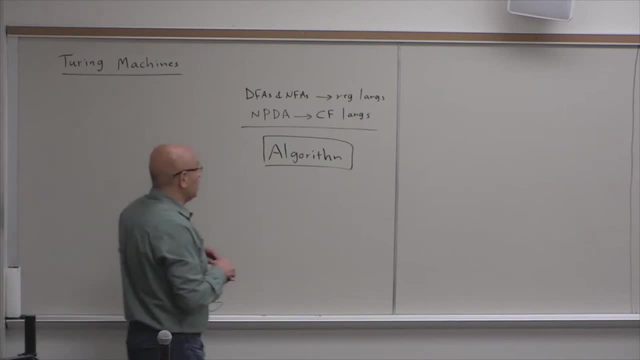 that not all problems are solvable using algorithms. Not all problems are solvable using computers, So we think of computers as amazing machines that can do anything. In fact, they cannot do anything. So there are things that computers cannot do There. 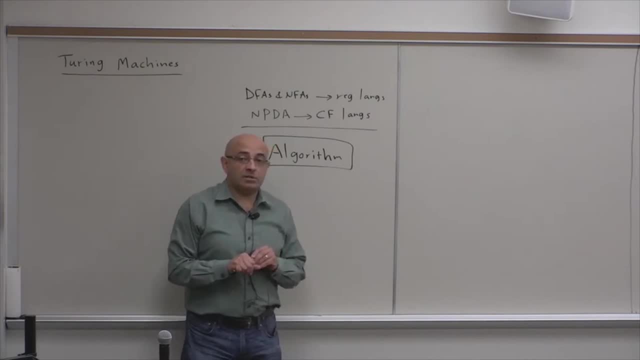 are problems that computers cannot solve. There are problems for which there are no algorithms. So why is that on the right side of the graph? Well, at the left side of the graph- And we will see this, you know- we'll understand this concept better. 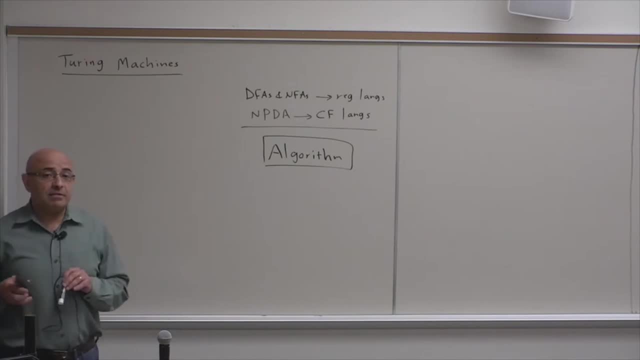 when we look into examples. Now let me just give a high level description of a Turing machine and how it, you know, differs from finite automata and push down automata, or how it's a more powerful machine. So clearly, in order for this Turing machine, 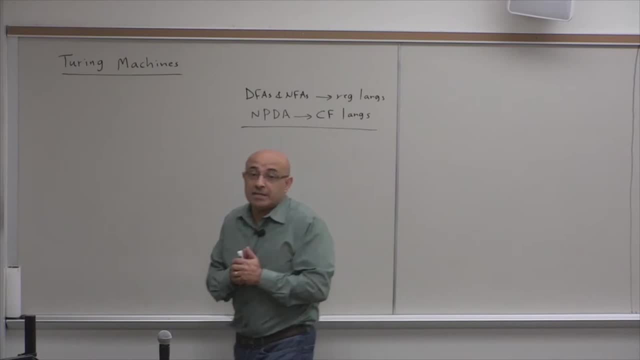 to recognize a larger set of languages. it has to be more powerful, And in order to be more powerful, it has to have more features that we don't have in finite automata and push down automata. Now let me ask a question. 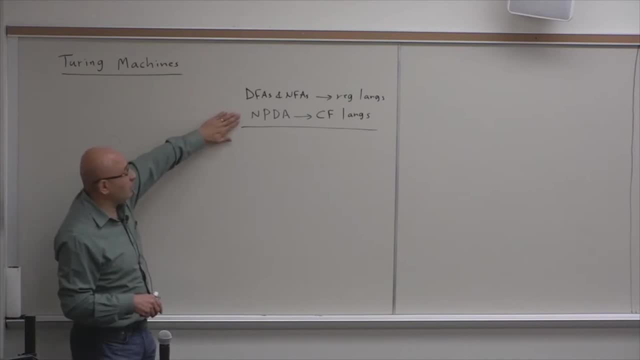 You know what's that feature that push down automata has, but finite automata? don't that allowed us to recognize a Turing machine, A larger set of languages? What's the feature that? what's that? The stack, yeah, So a push down automaton is more powerful than a finite automaton. 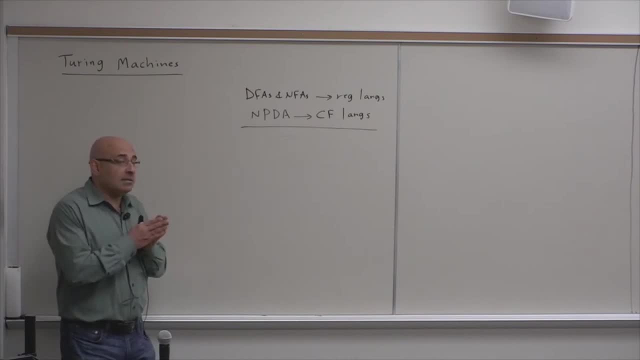 because it has a stack And that stack allows it, allows a push down automaton to remember things. its memory It's some kind of memory. Now, a Turing machine has memory, but it has a more more general kind of memory. 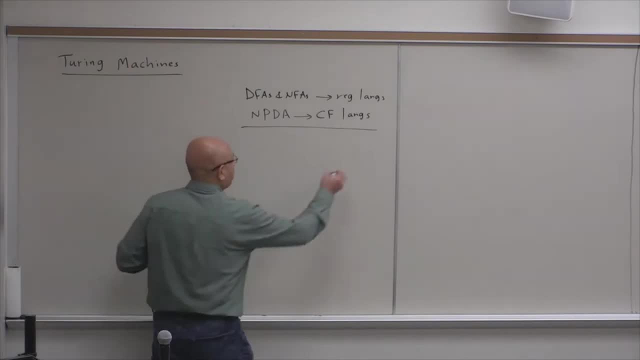 It has an unbounded tape. it has an unbounded tape on which it has the input. So the input can be A, B, B, C, A, So this is an input string And then on a Turing machine there will. we should have. 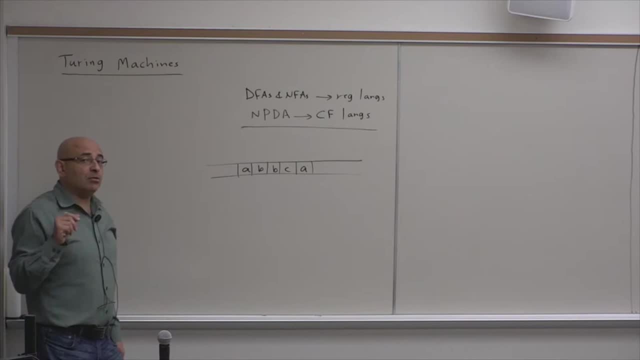 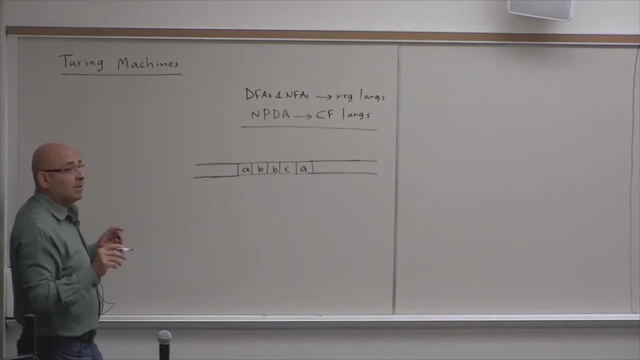 and the Turing machine is a theoretical model, by the way. So we're talking about a theoretical model. So this Turing machine is just a theoretical model for a general purpose computer. So this is infinite, but this Turing machine will have its head, the head of the machine, on this first symbol. 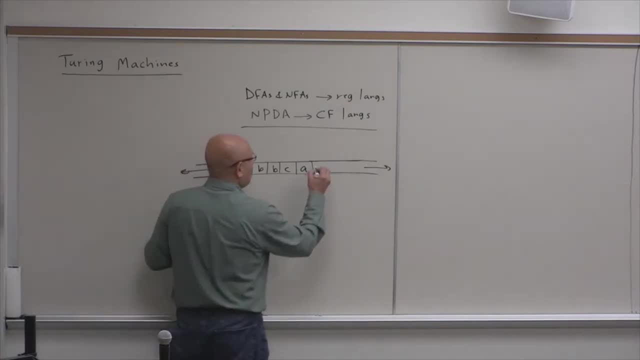 in the input string and there is some kind of another symbol, like the blank, to indicate or to mark the end of the string, And clearly this symbol cannot belong to the input alphabet Right, So it must be a distinct symbol. that does not belong. 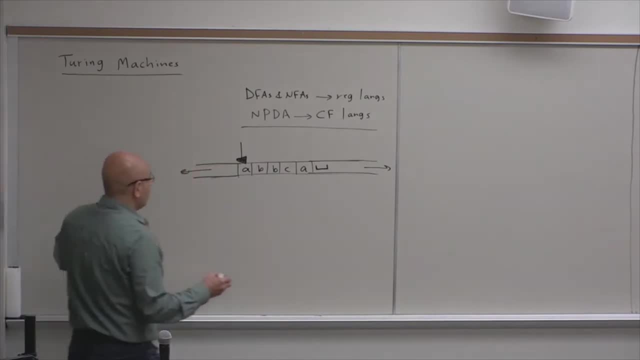 to the input alphabet. So these. so this is the actual string. So this is the actual string. The string has symbols that belong to the input alphabet that we call sigma, and in the Turing machine there is the tape alphabet that we call gamma. 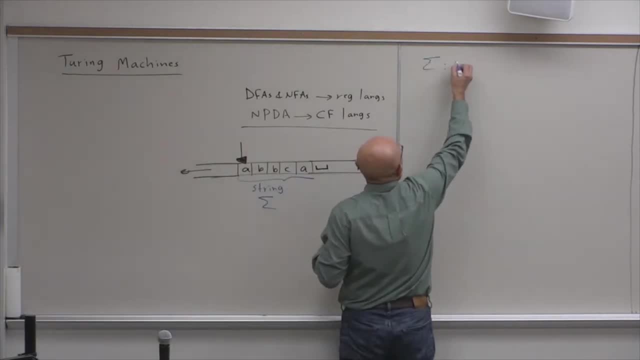 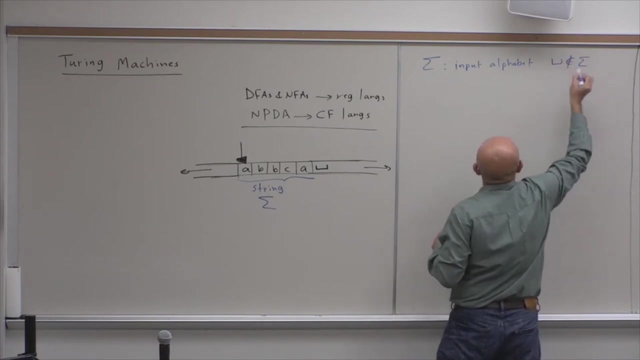 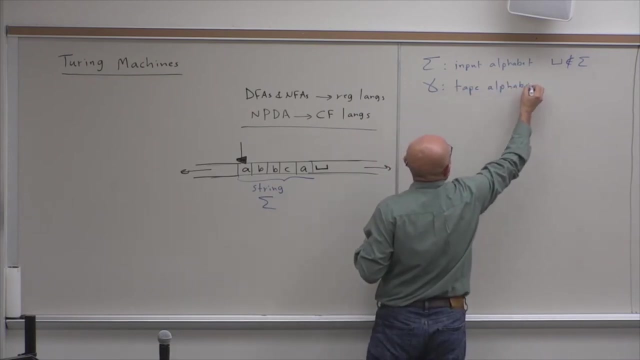 So sigma is the input alphabet and the, you know, this blank symbol does not belong to sigma and gamma is the tape alphabet and this symbol that marks the end of the string belongs to gamma, and sigma must be a subset of gamma. 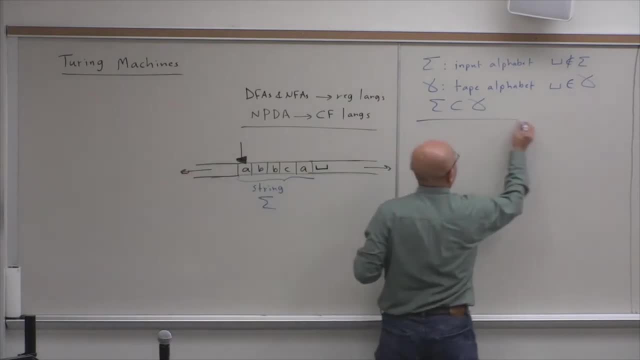 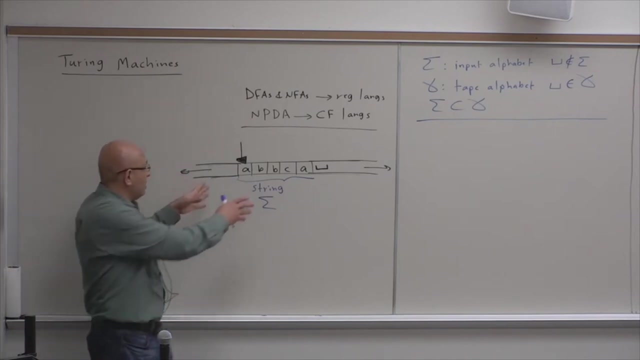 Sigma is a subset of gamma. Now, so far we have introduced a feature that the Turing machine has, but finite automata and push down automata didn't have, which is this unbounded memory. Now the power of the Turing machine is not limited, only 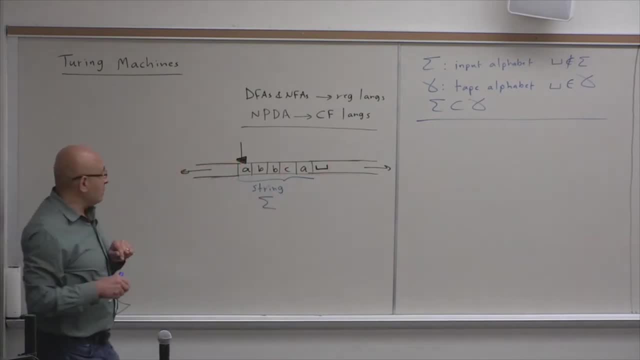 to having this unbounded memory. The power of the Turing machine. that distinguishes a Turing machine from the less powerful Turing machine, the less powerful automata- is that it can read and write. So it doesn't only read from the input, it can also write. 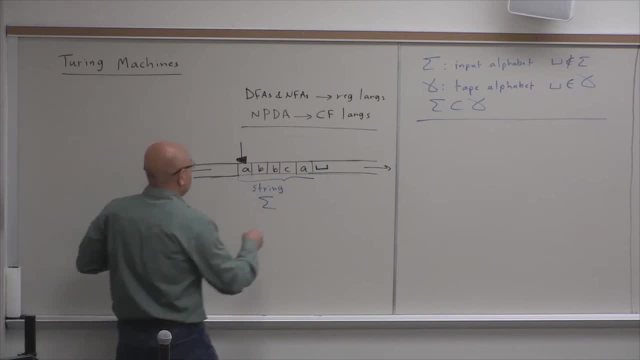 So it can choose to replace this B with a C, for example. So a Turing machine not only reads from the input, it can read and write. And this head of the Turing machine can go left and right. So This head can go right and it can also go back to the left. 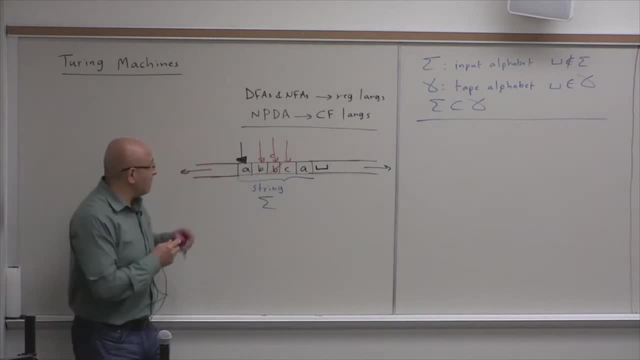 So if the tape of the Turing machine, if the head of the Turing machine can go left and right, this means that a symbol in the input can be processed multiple times. And this- the fact that you can process a symbol multiple times- it makes the Turing machine more powerful. 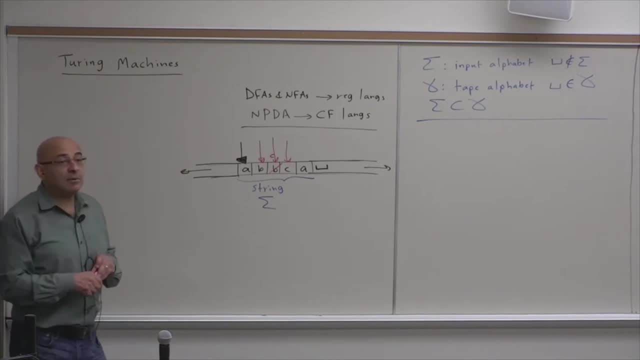 but also makes it more complicated, Because now a Turing machine is not guaranteed to terminate within finite time. Finite automata and push-down automata are guaranteed to terminate within finite time because the input string is finite And each symbol in the input string is processed only once. 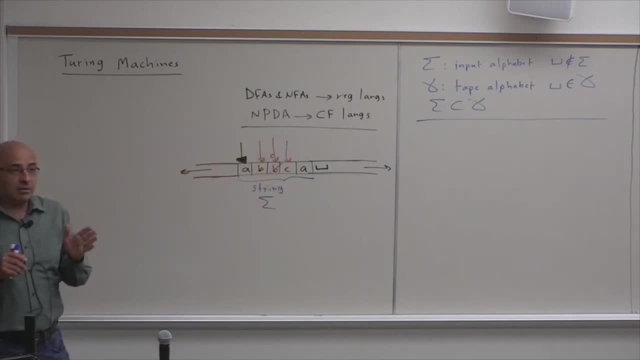 It's touched once. So finite automaton or a push-down automaton touches a symbol in the input string only once and the input string is finite. Therefore, a finite automaton or a push-down automaton are guaranteed to terminate within finite time. 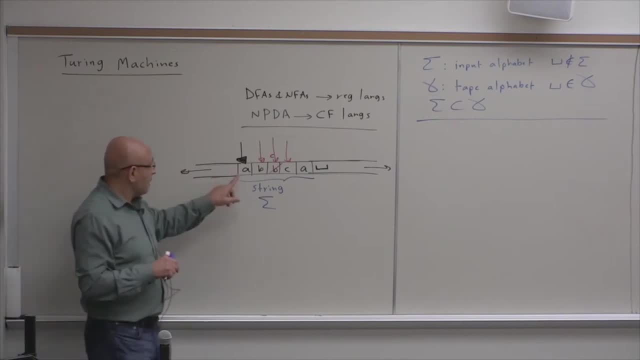 Now in a Turing machine. the Turing machine can process or can touch each symbol multiple times, An unlimited number of times, which means that a Turing machine may not terminate within finite time. So the Turing machine, the extra features in the Turing machine, 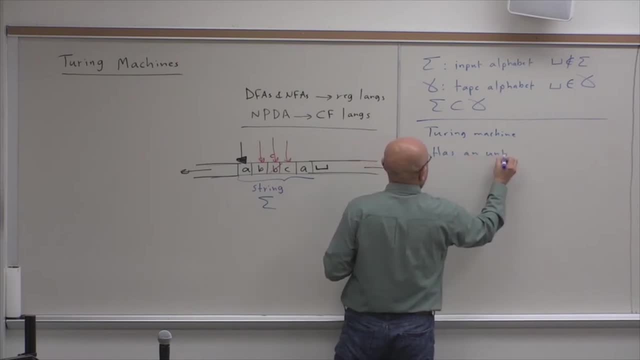 has an unbounded tape or you know memory, Which is memory. It can read and write and it can go left or right, Which implies that an input symbol, in fact, when it goes left and right, it doesn't have. 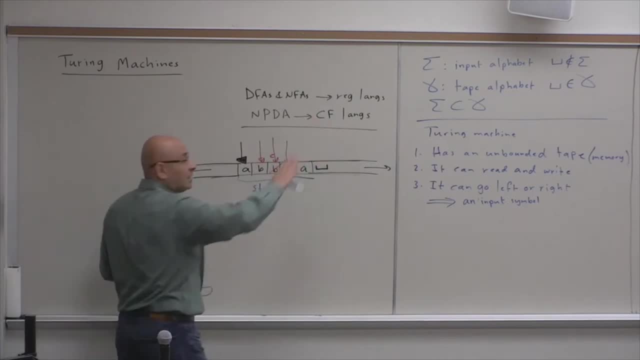 to process an input symbol So it can go beyond the input string. So this is in this example: we have an input string with five symbols in it. The Turing machine can go beyond that, Can write its own symbols beyond the input symbol. 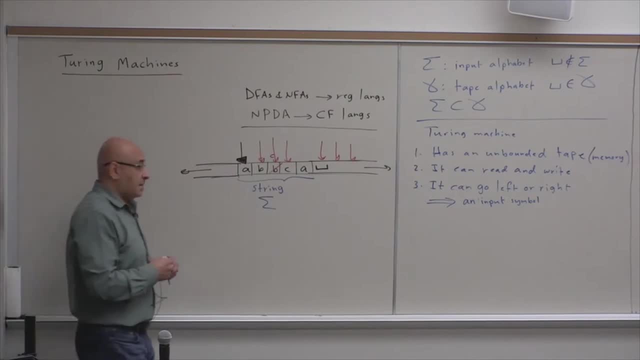 So you know, just like you know a computer program that we are familiar with, Your computer program reads. you know a certain input, There is an input to your program, But your program also writes, And it also. it can you know. 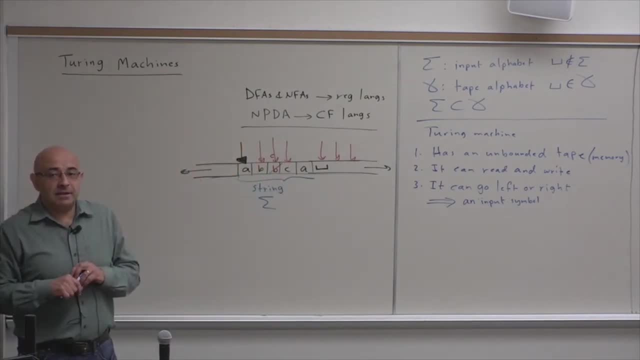 it can read the input. You know, generate all kinds of data structures in memory. So that's you know what you have in memory at any given point. can you know greatly exceed what you have at the input? You know what the program writes in memory can be much. 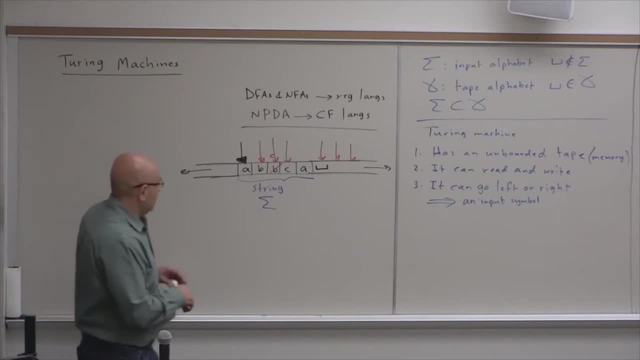 much more than what you know the input is. So this is. you know. we are going now to a more, much more general model of computation. So an input symbol. The input symbol may be processed multiple times, So a Turing machine. 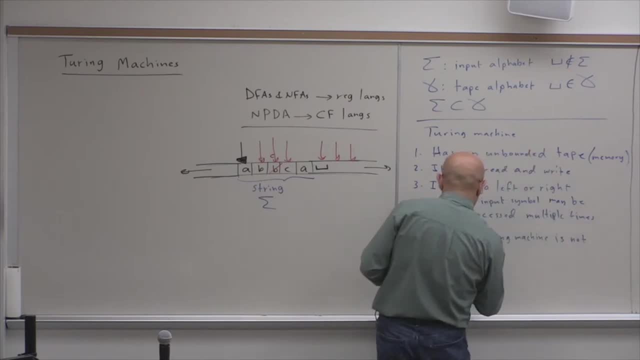 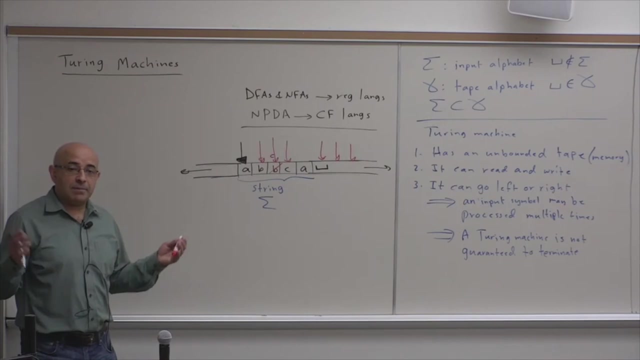 Is not guaranteed to terminate. So, just like a general program, a program written using a general purpose programming language may not terminate. It may have infinite loops, It may have infinite recursion, It may have recursion without a base, And then it will never terminate. 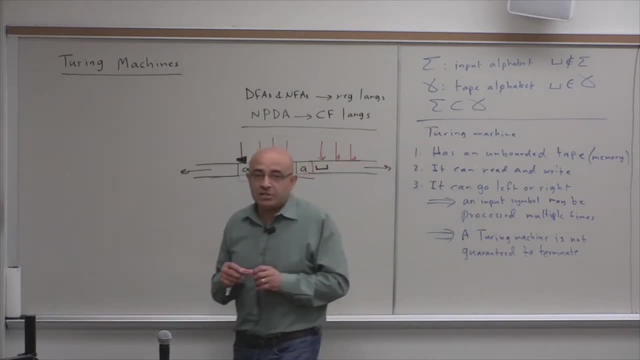 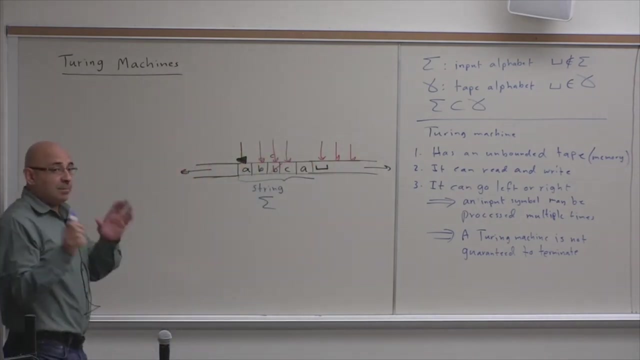 So you know, termination is not guaranteed. If you're not, every algorithm is guaranteed to terminate. Now this introduces the concept of decidability versus recognizability. So a Turing machine, because the Turing machine can have given an input string. in a Turing machine, now you can have three. 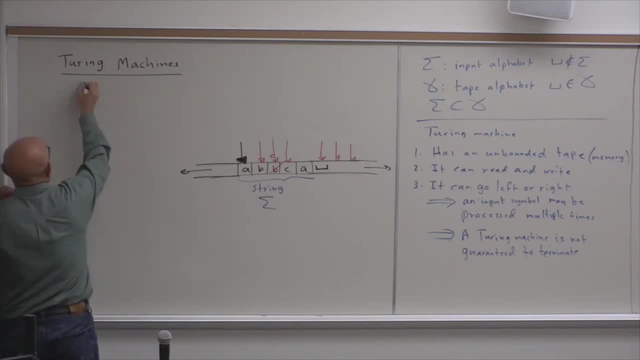 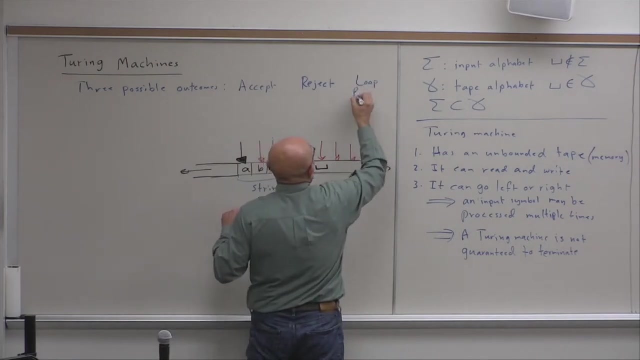 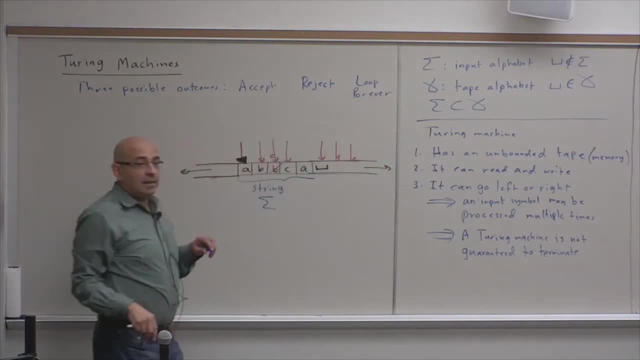 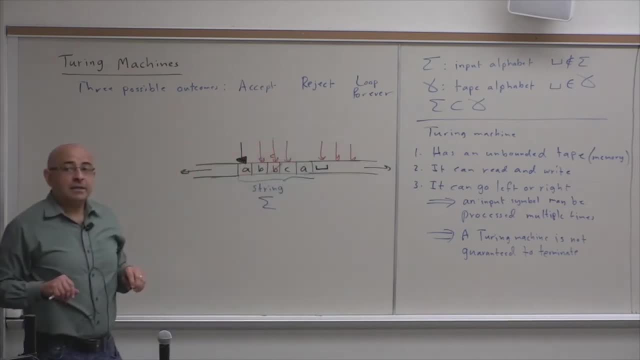 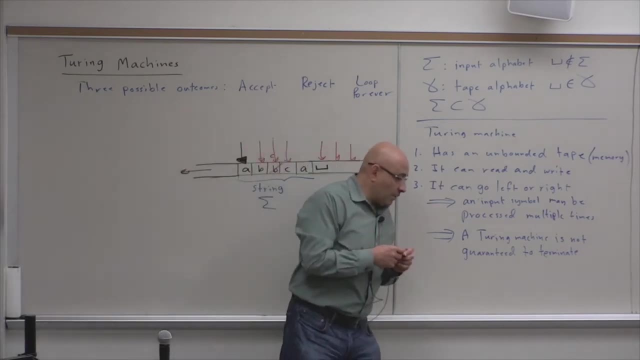 And this loop forever is not there Because, by definition, when we describe the input it's you always make you know you have to process the input string And with an input string it's you have to process the symbols of the input string. 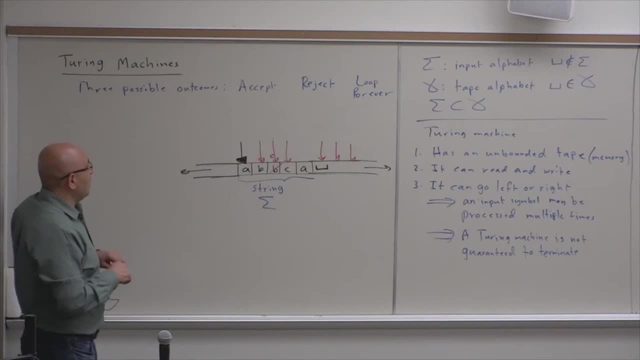 And if you end up in an accept state, that's an accept. If you end up in a reject state, then you reject. So now we have the notion of decidability versus recognizability. So if a Turing machine, if a Turing machine ends with an accept, 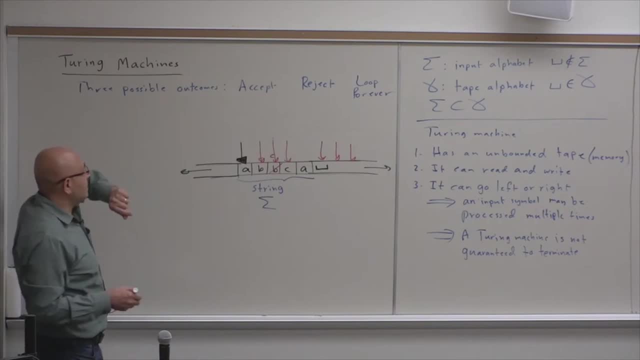 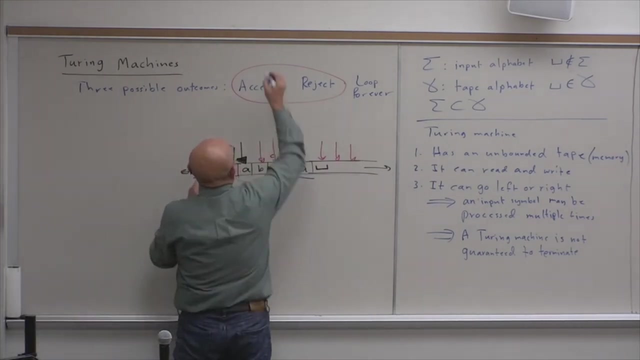 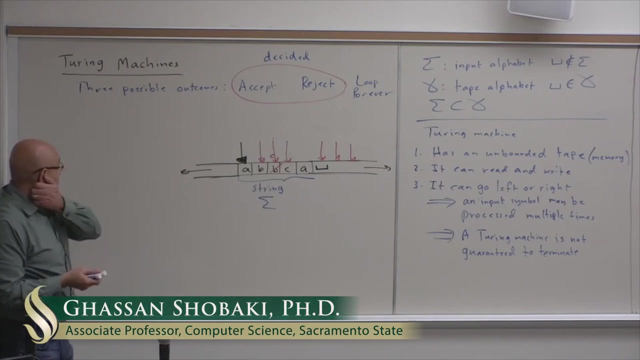 or reject, we say that the Turing machine has decided the input string. So if the outcome is accept or reject, we say that this input string has been decided. Or in other words, if, for a given language, you can find a Turing machine that will either accept or reject, 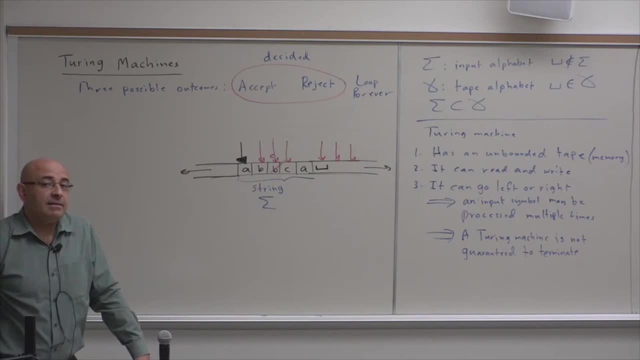 and is guaranteed not to loop forever, then you say that this Turing machine decides this language. So if, if the Turing machine decides the input string, then you say that this Turing machine decides the input string First, I have to conclude that if a eğ is coming from a Mi problem. 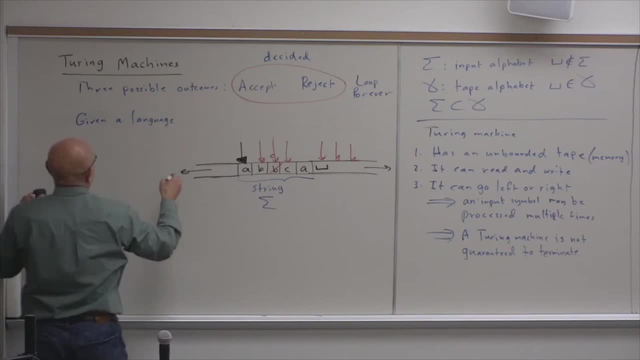 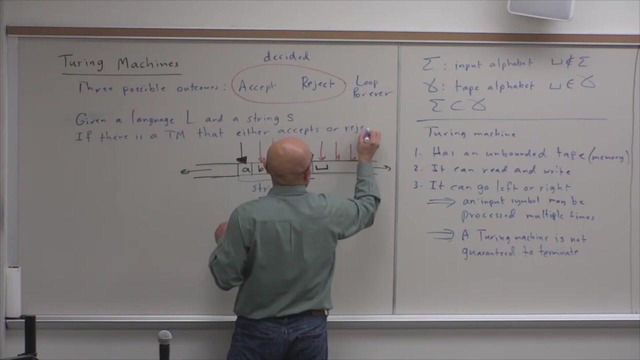 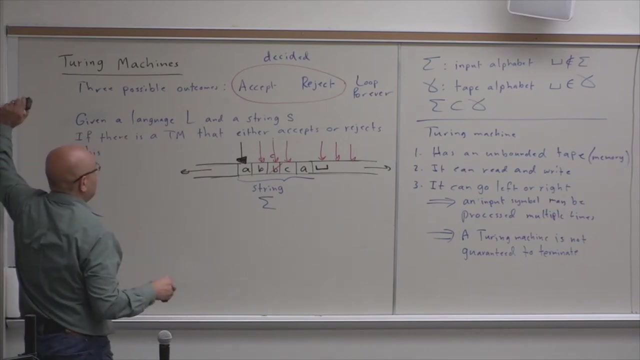 if the Turing device, if, or a language, if a Turing machine decides the input string and is not accepting or reject Turing machine, that is void from Turing that either accepts or rejects, That either accepts or rejects this string, the given string, in finite time. we say that the Turing machine decides. 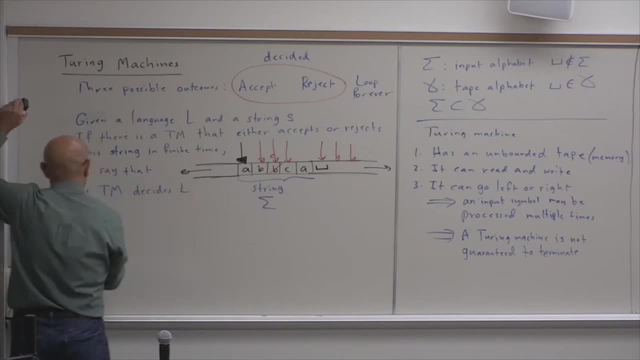 whether a language is Turing-decidable or L is Turing-decidable. L is Turing-decidable. So a language is Turing-decidable if you can find a Turing machine that will either accept or reject. Now, if we change the Turing machine, 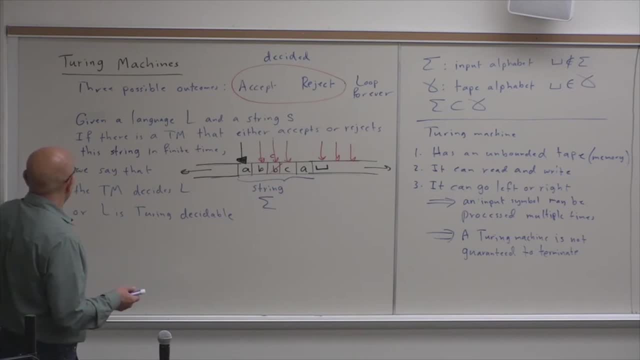 if we change this definition, given a language L and a string S, if there is a Turing machine that accepts S, if S belongs to the Turing machine, then the Turing machine will accept the Turing machine. Okay, Okay, Okay, Okay, Okay. 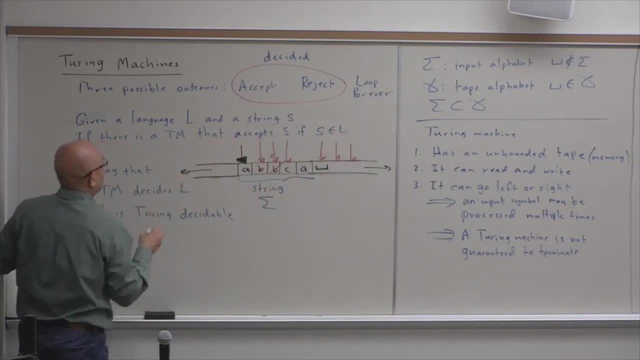 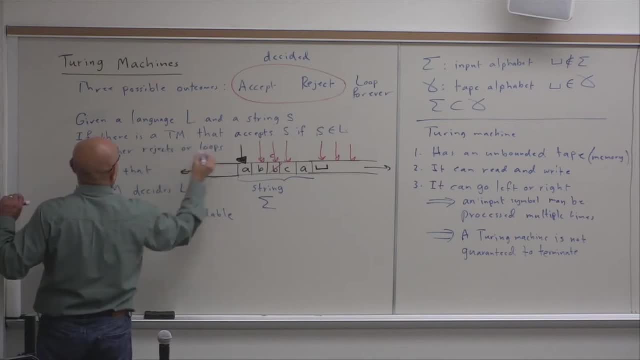 and either rejects or loops. If S does not belong to the language, we say that the Turing machine recognizes S And L is Turing recognizable. Okay, So do you see the difference between decidability and recognizability? So if you can find a Turing machine that will either accept, 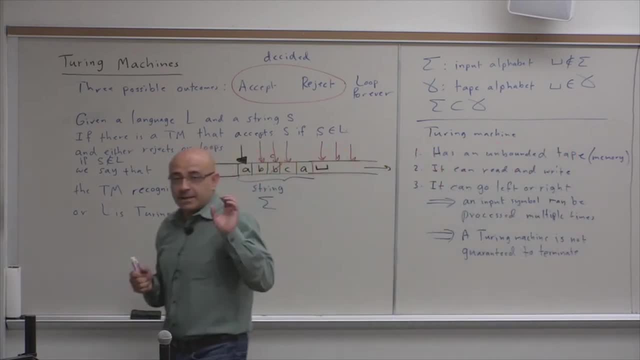 or reject within finite time. it accepts every string that belongs to the language in finite time and rejects every string that belongs to the language in finite time. We say that the Turing machine decides the language. If we don't have a machine that decides the language, 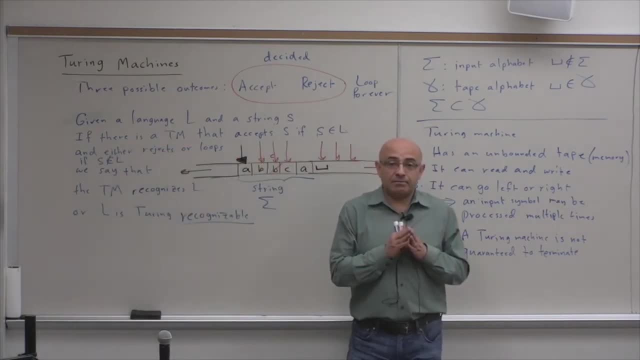 we have a machine that if the string belongs to the language, it's going to say it's going to accept it. But if the string does not belong to the language, the machine will either reject it or loop forever. So if the string does not belong to the language, 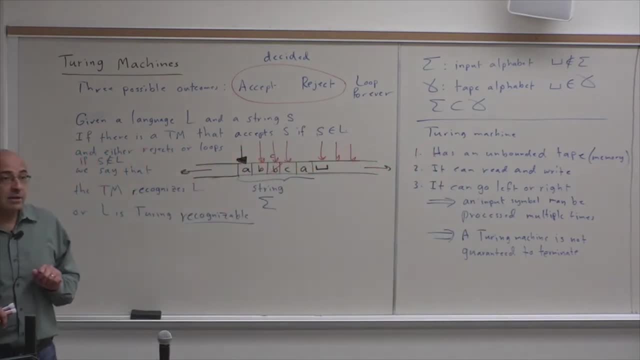 the machine is not going to accept it. It's not guaranteed to terminate within finite time. In this case, we say that the Turing machine recognizes that language. Now, given this description, which set is larger: the set of Turing decidable languages or the set? 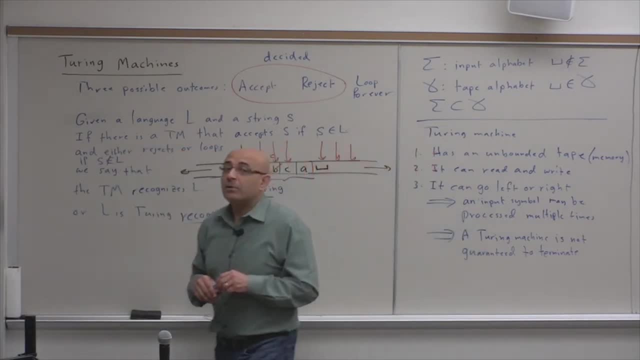 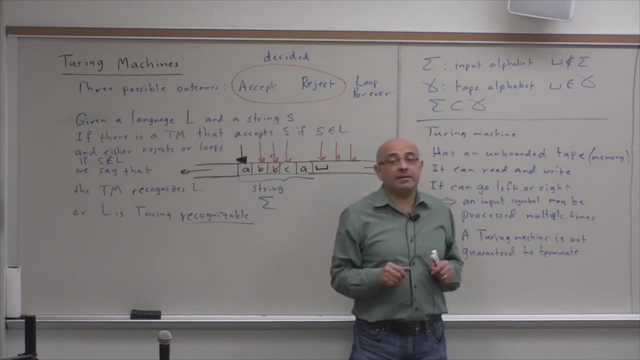 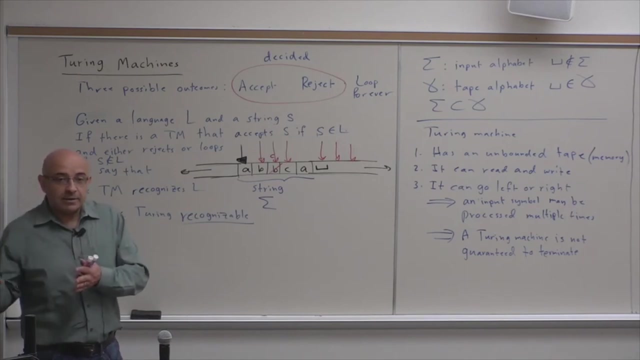 of Turing recognizable languages, Which one will be larger Recognizable? Yeah, exactly Because recognizing is easier than deciding, Right? So if a language is decidable, it's recognizable, Because here recognizability it's if the string belongs. 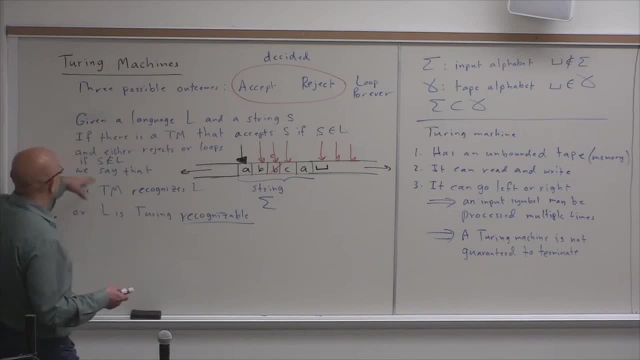 it accepts it. If it does not belong, it either rejects or loops, So it doesn't have to loop Right. So if a language is decidable, every decidable, every recognizable language is recognizable. but the opposite is not true, Of course. you know, we will show, you know, this lecture. 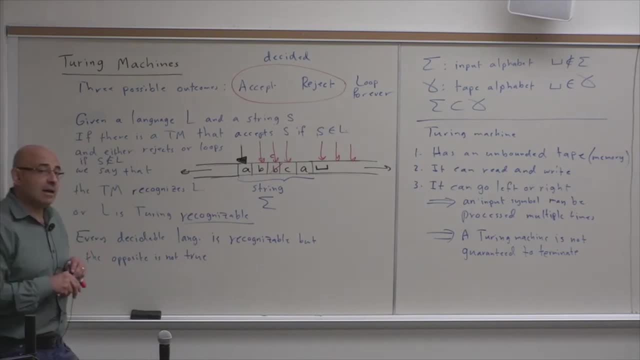 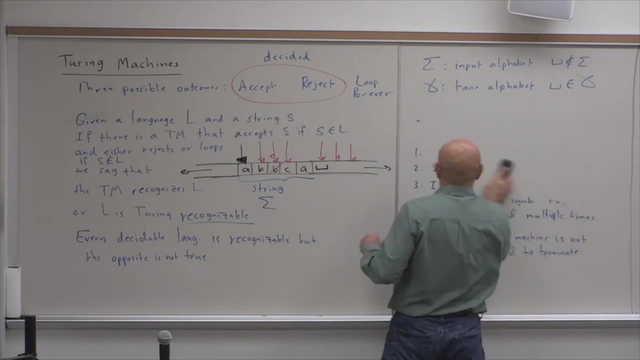 and in next lectures we'll show examples of decidable and recognizable languages and you know, with the examples, you will, you know, fully understand the concept. So now, let me, after you know introducing this, let me draw the hierarchy now of languages. 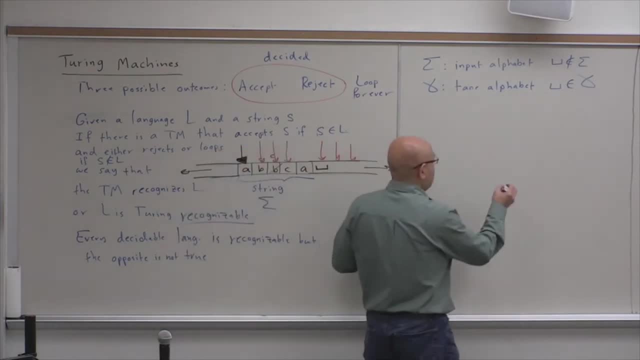 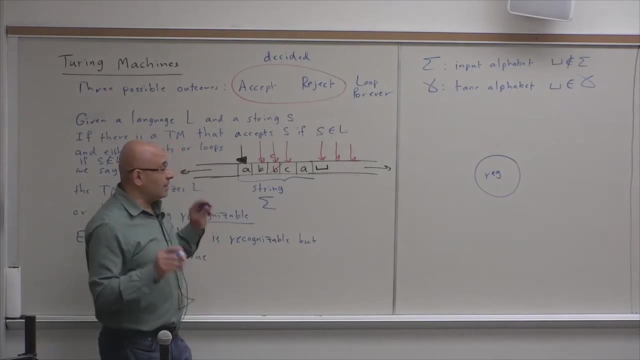 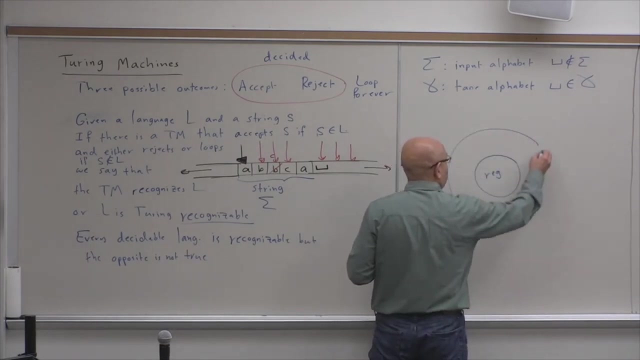 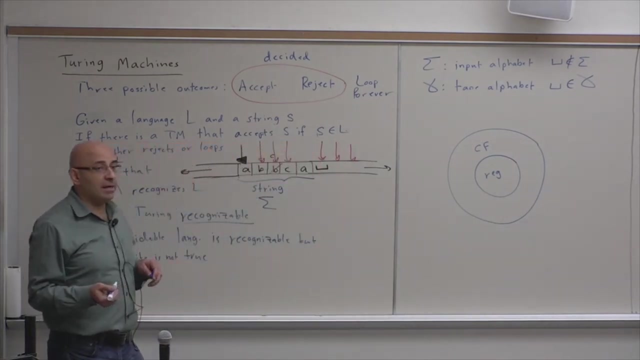 So I have, we have the smallest set that we started with, which is regular, regular language. These are the languages that can be recognized using a finite automaton. And then we introduce the set of context-free languages, The set of languages that are recognized by. 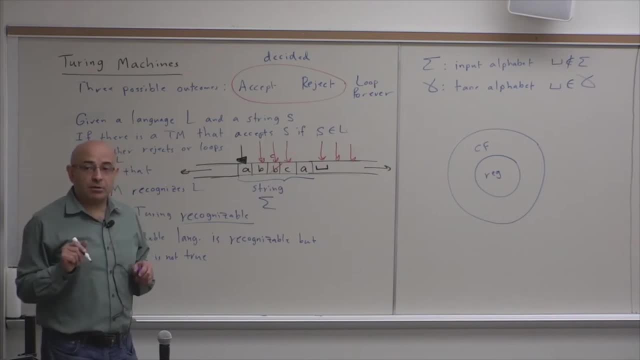 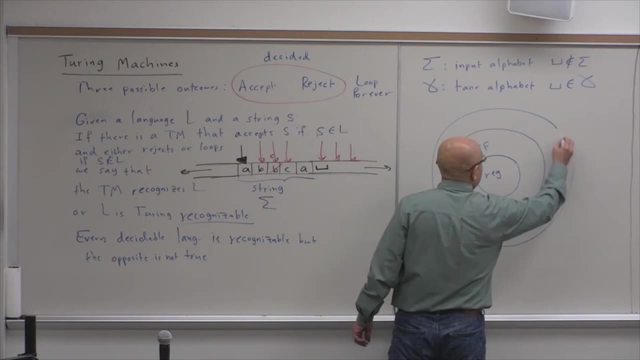 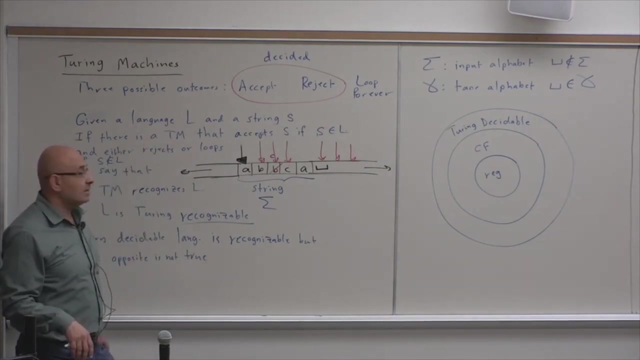 that can be recognized using non-deterministic push down automata. And now we have a larger set of languages, which is the set of Turing decidable. You know, the Turing machine is more powerful and it can decide a larger set of languages Turing decidable. 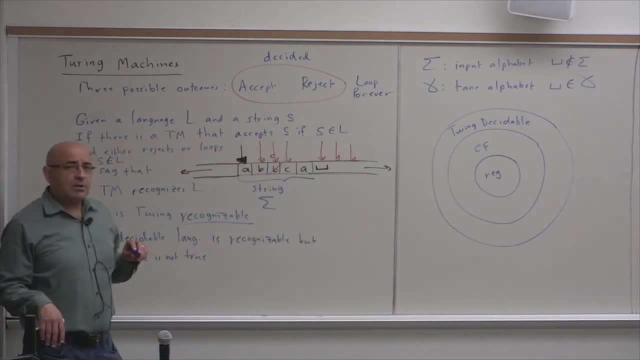 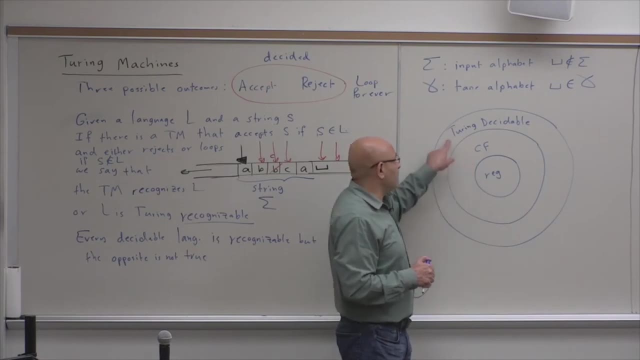 You know now. we know that. you know. it's just. you know, if a language is context-free, it's clearly decidable. Why? Because a Turing machine is more general than a push down automaton And a Turing machine is more general than a finite automaton. 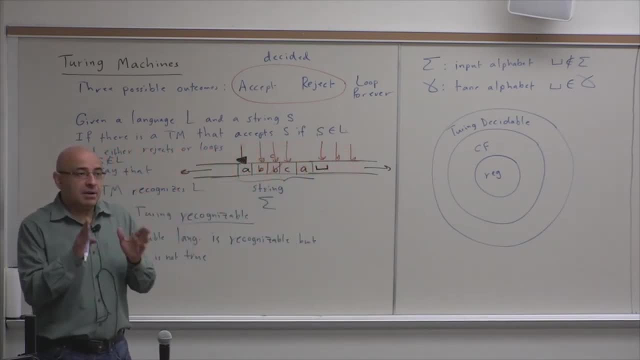 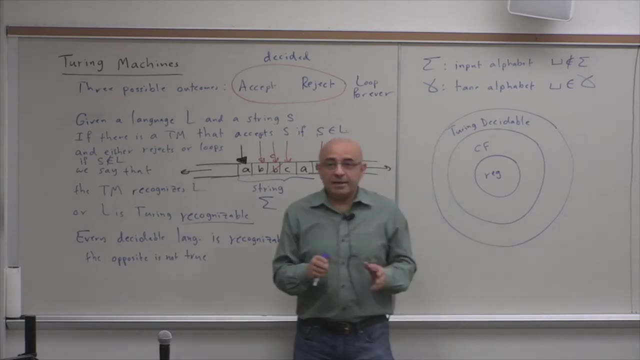 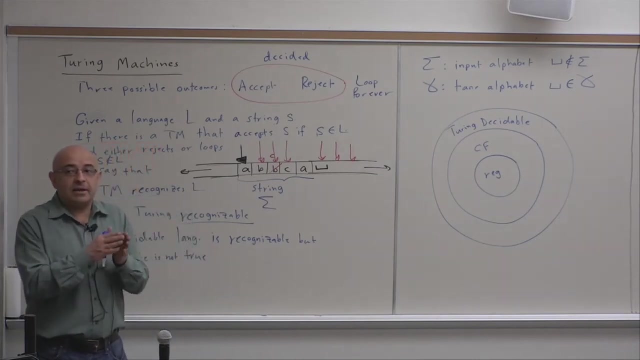 So a Turing machine can easily simulate a push down automaton and it can easily simulate a finite automaton. It's just, you know, when it simulates something that is less powerful, basically it's using fewer features, So it has more features. 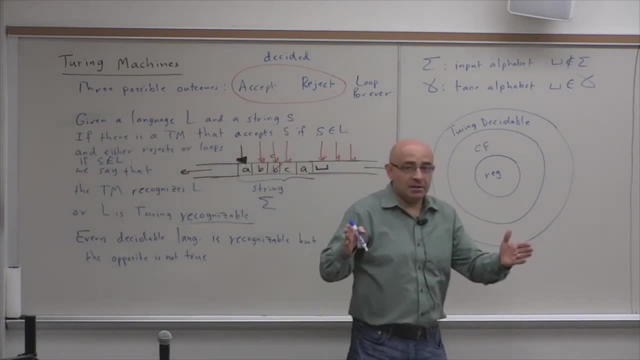 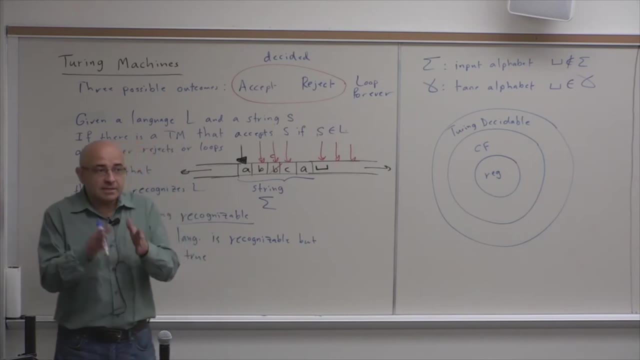 The Turing machine is more general. It has more features, So when it simulates something, to simulate something that is less powerful, it just uses a subset of the features that it has. Okay, so it's easy for the more powerful machine to simulate the less powerful machine. 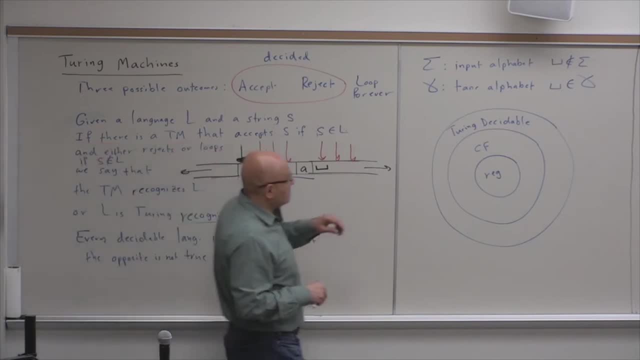 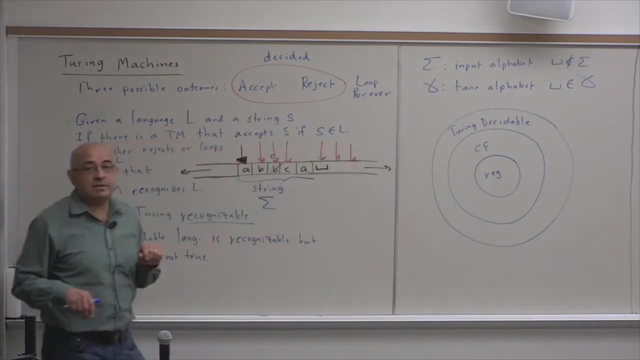 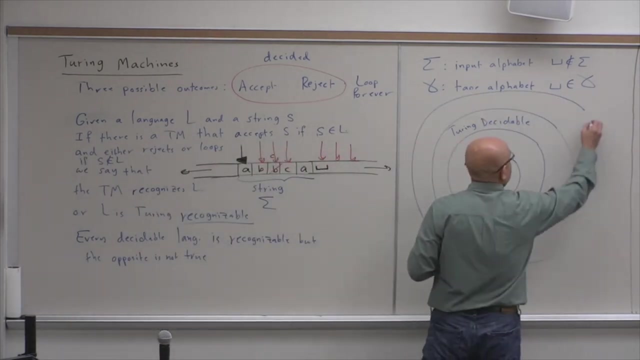 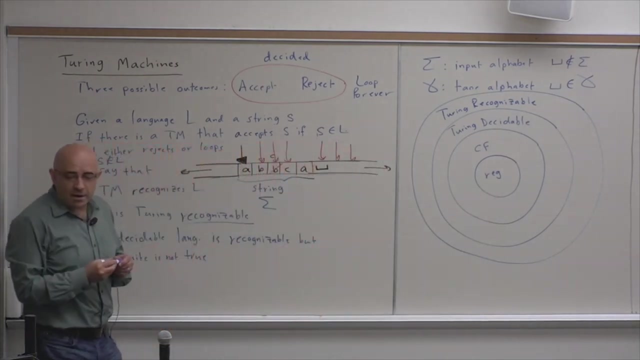 So that's why the set of regular languages is, and context-free languages is a subset of the set of Turing-decidable languages, And the set of Turing-decidable languages is a subset of what Turing-recognizable. Okay, so there are other names, equivalent names. 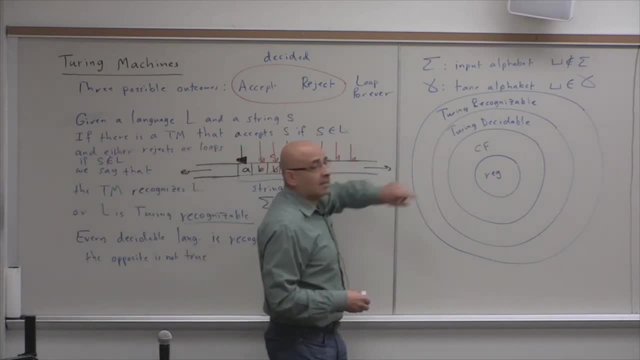 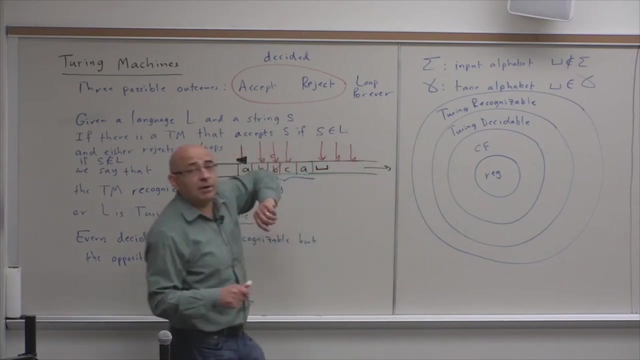 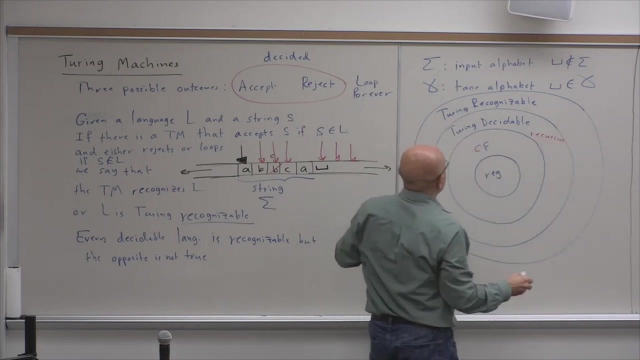 or alternative names for these. So Turing-decidable languages are called enumerative languages and this is called recursive languages, and this is the set of recognizable languages is called recursively enumerable languages. So this is recursive and this is recursively enumerable. So these are alternative names for Turing-decidable languages. 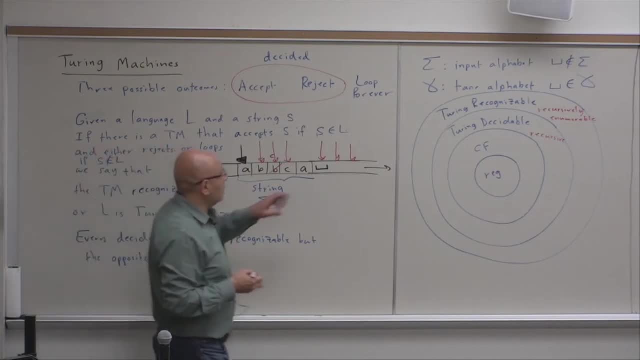 that are also called recursive languages, and Turing-recognizable are also called recursively enumerable languages. Okay, so now let's give a high-level description of a Turing machine that will recognize, or that will decide, in fact, one of the languages that we have. 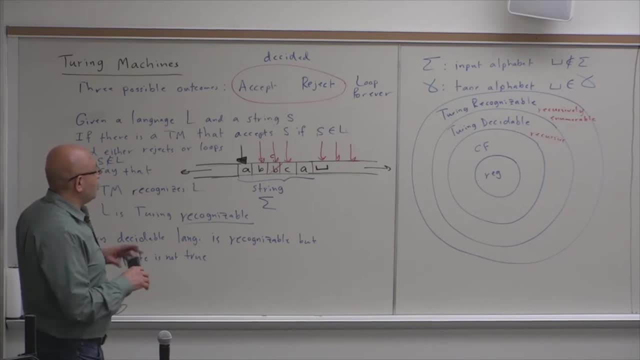 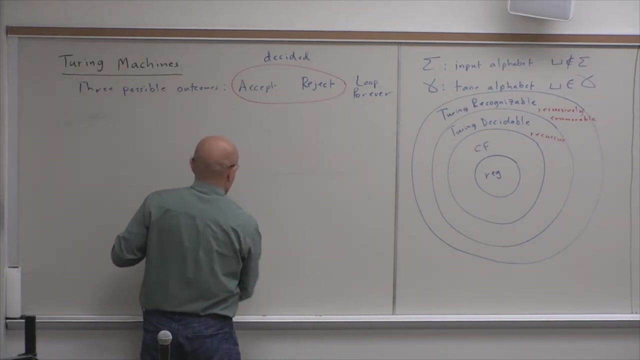 have studied and shown to be non-context-free, So let's give a high-level description. By the way, a state diagram for a Turing machine is going to be messy and we will only see an example of one small, only one small example for one language, for the state diagram. 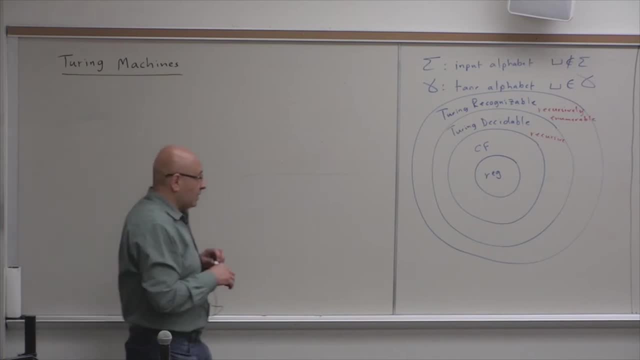 for a Turing machine because it's messy. But most of the time we will give a higher-level description of a Turing machine, not a complete state diagram For this case. so let's look at this example. L is W pound W, such that W belongs to sigma star. 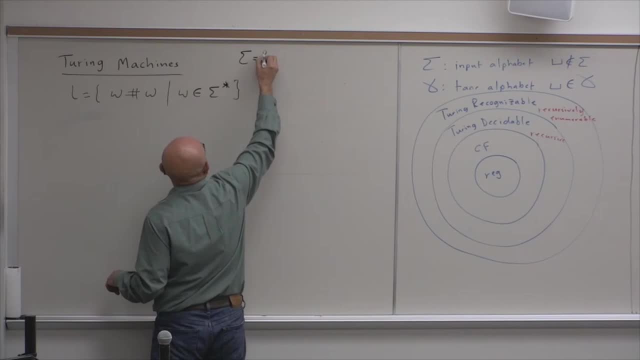 and sigma star is, let's say, 0, 1.. Sorry, sigma is 0, 1, and W belongs to sigma star. So this is W separator, some kind of separator? W. Now, this is a language. 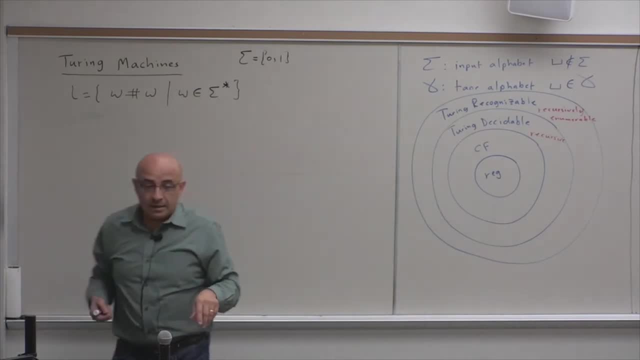 This is a language that is not regular and it's not even context-free. So last time we showed a language that is similar to this, looks similar, that is context-free. and what was that? Yeah, the palindrome. So W W R is context-free, but W? W is not context-free. 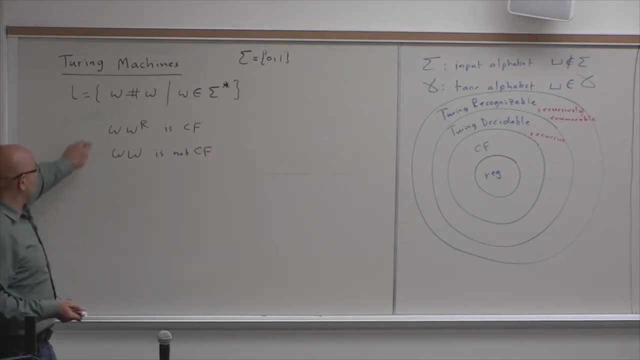 So you know, it's easy to write a grammar for this, but if you try to write a context-free grammar for this, you will not. You will not be able to write a context-free grammar Because, if you know, think about it for the palindrome. 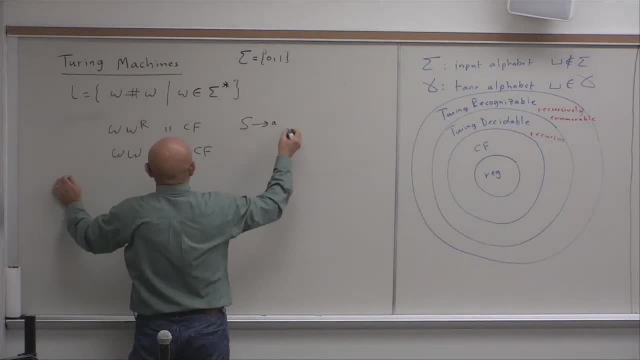 you wrote this. you wrote this grammar: A, S, A or B, S, B or epsilon, and this is this- guarantees that you know you have this kind of symmetry around a certain axis. So for this we could write a context-free grammar. 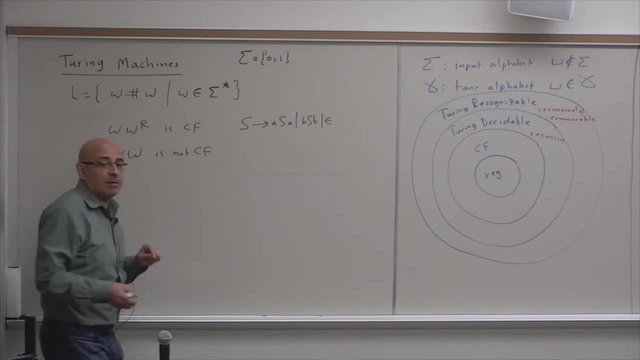 but try to think, try to write a context-free grammar for this. you will not find a way. So you cannot say something like this: S is, for example, you know S1, or you know AA, for example. 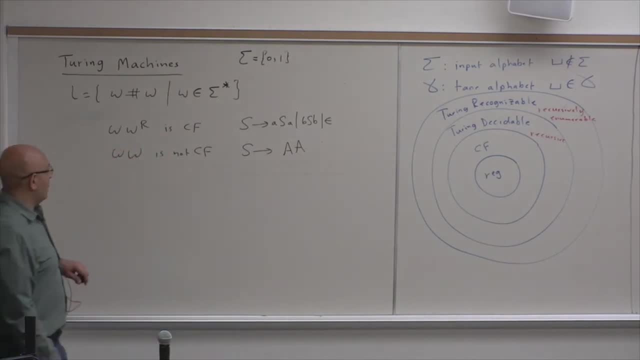 An attempt would be: S is AA and then A is anything, or BA or epsilon. Will this generate this? No, it will not generate this. Why? Because what you use for there is nothing that will force this A to be the same as this A. 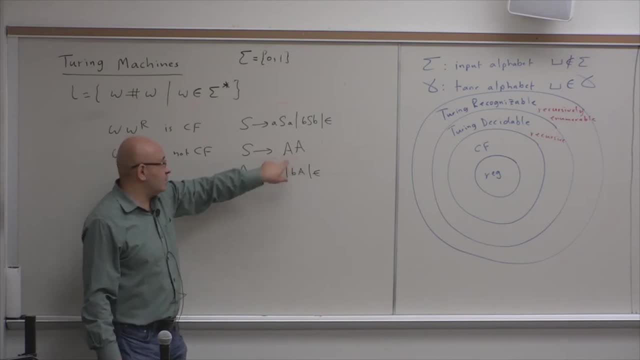 So this is an arbitrary string and this is an arbitrary string and these two A's can be different, Right? So this is just a naive attempt to construct a context-free grammar for this, But there is no such grammar because this language is not context-free. 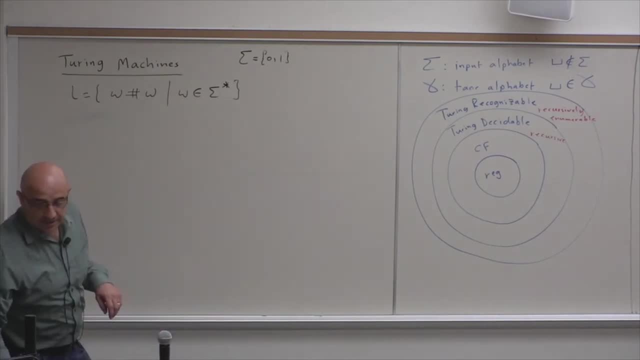 Okay. So now how does the? let's show by example how a Turing machine can recognize this language. So let's look at, Okay, So let's look at this example: One zero one, one, zero one, Okay. So this is the input string and this is the Turing machine. 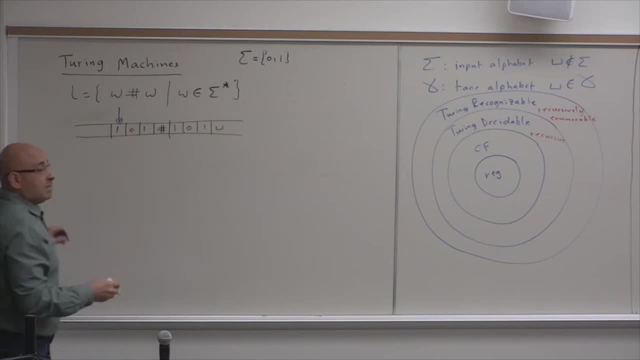 So this is the head of the Turing machine. Now the Turing machine can go left. you know, the head can go left and right and it can also write. So the algorithm for recognizing this is checking if the first symbol matches the first symbol after the pound. 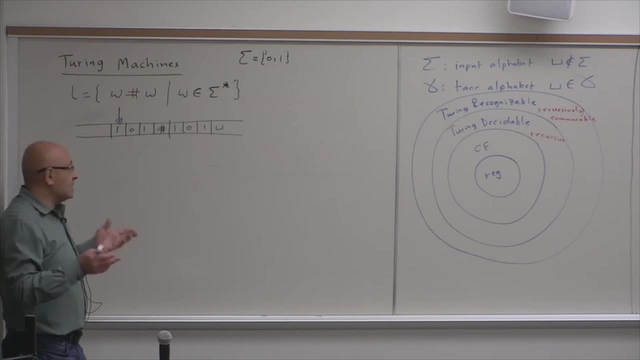 and the second matches the second after the pound. So you can do this in a systematic manner by using crossing. So you can say, okay, at this symbol, I'm going to cross or mark this one, I'm going to mark it. 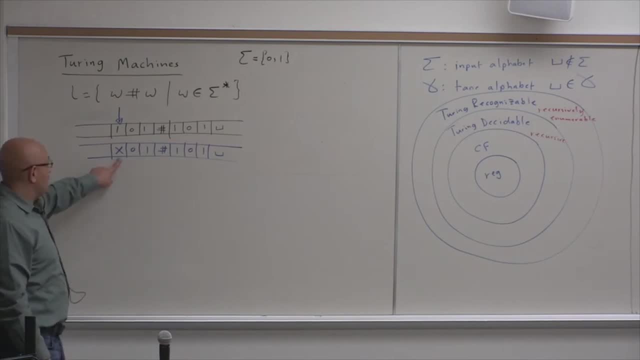 Mark this, you know, to indicate that I'm done with it, And then compare- you know, the symbol that I have just read. then the head goes right until it finds the the pound sign or the symbol that indicates that separates the two parts of this string. 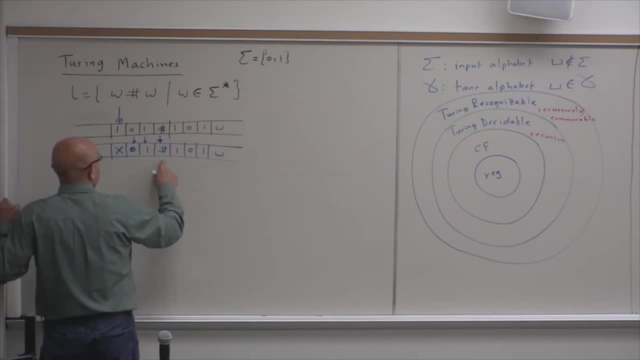 And then it- you know it- checks the first symbol after this: Is this equal to the symbol that we have crossed? If it's equal, then we are still. then the test passes and the string so far satisfies the property of the language. 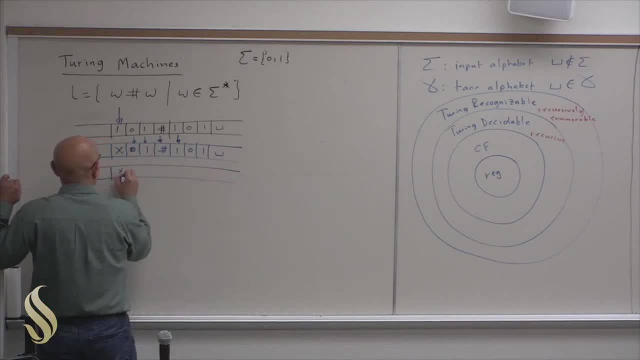 So it's going to do this, It's going to mark this, And then now we have marked this and this after matching them, And in fact, you know, the Turing machine can keep doing this. So now, if the head is here, 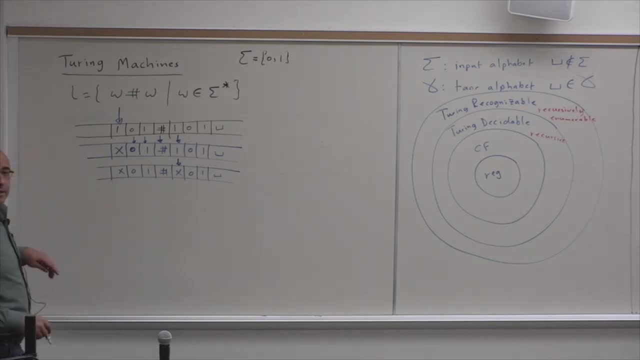 now the head will be in the same position. So now the head will go left. So you keep going left and checking until it finds what. Until it finds, No, it doesn't know. it will not stop here because it will not know that this is the first unmarked symbol. 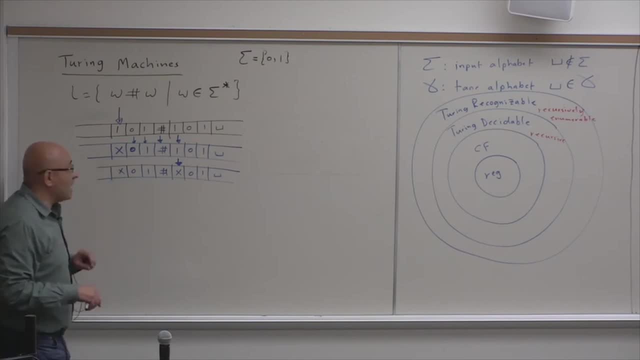 It has to go all the way to the X to find the last marked symbol. So it will have to go all the way to the left, one step at a time. So each one is going to be a transition, you know each. 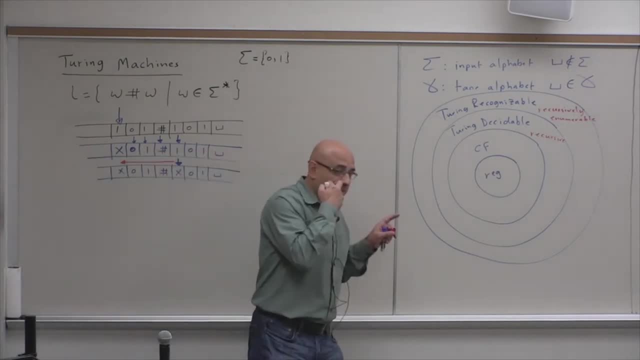 So that's why you know, our description of the Turing machine here is high level and we are not showing all the details. So the head will get to this X one step at a time. So each time it will go one step to the left and it will check. 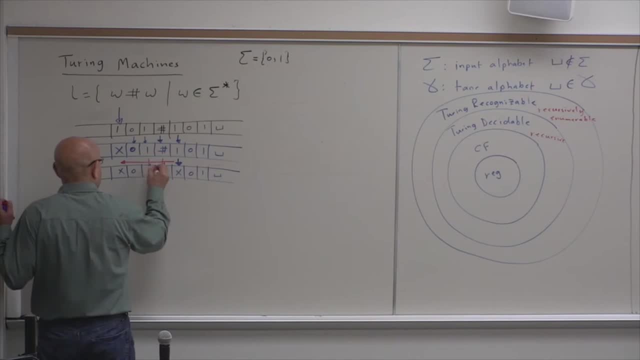 Is this an X? No, it's not an X. Go to the next. Is this an X? No, it's not an X. Go to the next. Is this an X? No, Is this an X? Yes, So it will keep going and checking if it's an X or not. 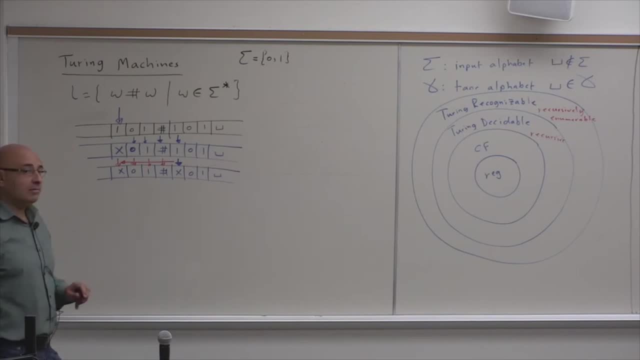 Now it's an X. When it finds an X, what should it do? It should go right. If it finds an X, it should go right. and now this is our next symbol to check. And it's a zero, So it's going to mark it. 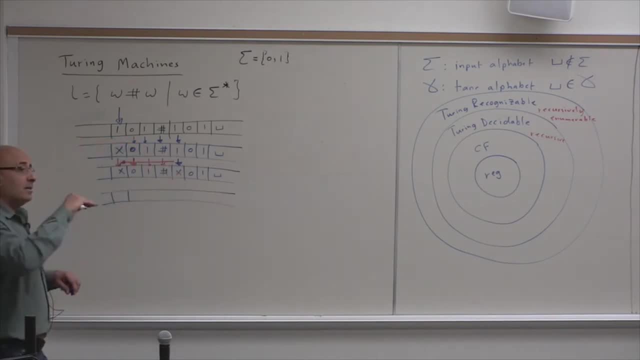 Now, each line here that I'm drawing does not represent one step. It has multiple steps. It has multiple steps in it, as we have seen. So this is an X, So it's going to mark this, and then it will go to the one pound X, zero one. 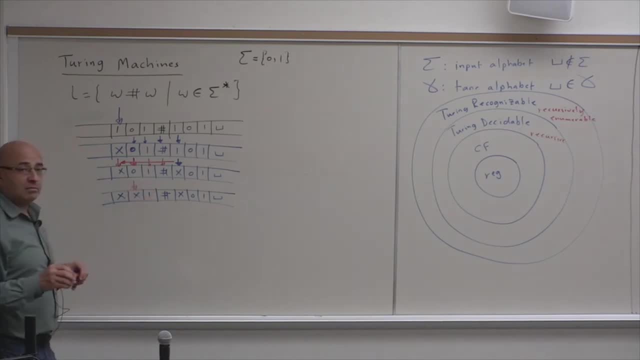 Now we are here. Now what should we do? So this tape should go right until it finds a what Zero? No, It doesn't know if it's looking for a zero or a one. Yeah, It needs to go for the X. 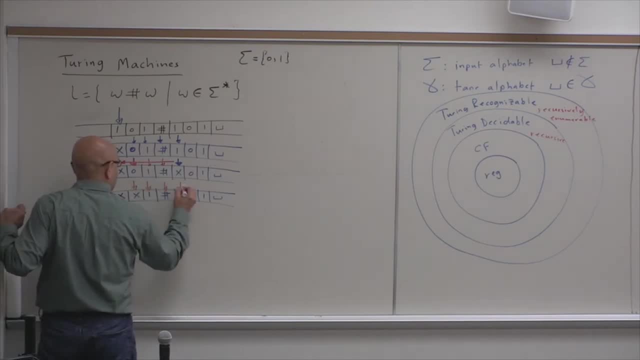 So it should go one step at a time until it finds an X. Then it checks, So then it goes to this zero. So whatever the symbol after the X is gets compared with the last marked symbol. So this should match this, And if it matches, then it's going to mark it with an X. 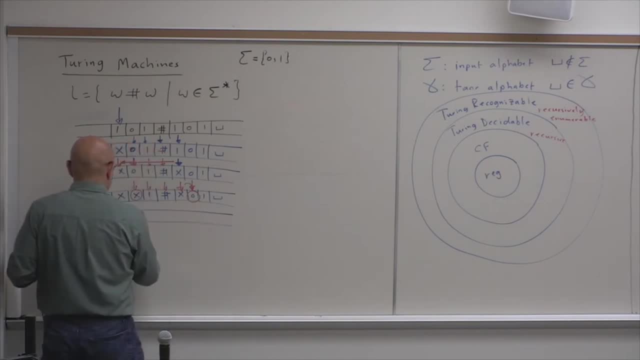 You know what I'm saying? It's going to mark it with an X. It's going to mark it with an X. Okay, You know so clearly. this is tedious, but it works. So this is X one, And then it's going to do the same. 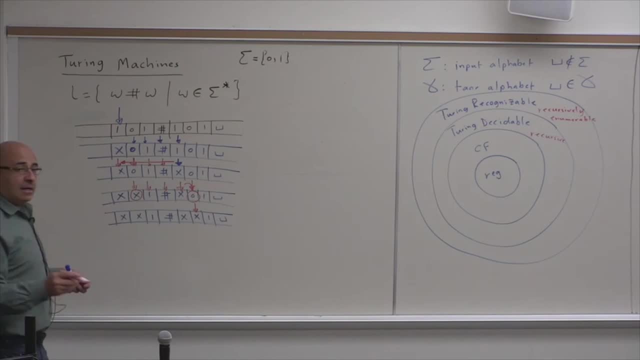 So we are here. It's going to keep going left, so that this head will go left one step at a time until it finds an X. Then it looks at the symbol, then it goes right. So it keeps going left until it hits an X. 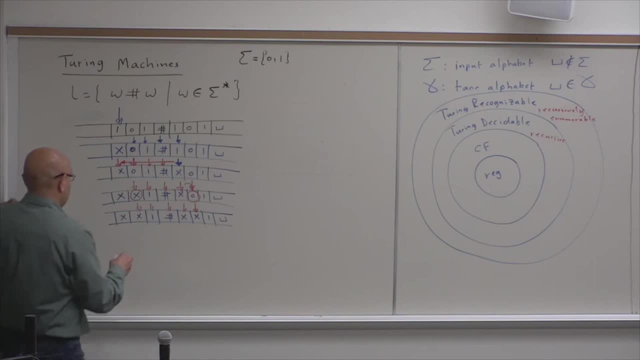 Then it goes right. What comes after the X is this: It says: okay, now this is the next symbol to match. It marks it with an X and goes right. And again I'm skipping many steps, And now it's here. 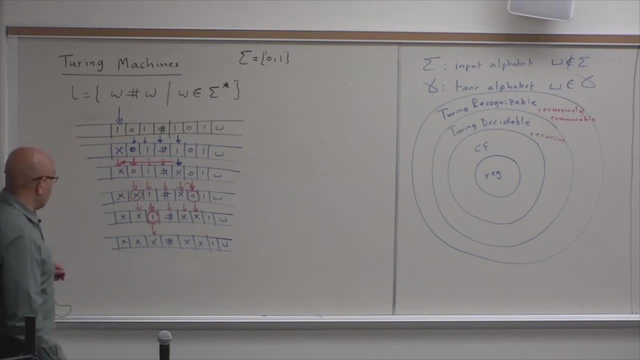 The tape is here, Then it goes left, Then it goes right- sorry- until it finds the last X, right. So what we should be looking for now is the last X. So X, X, X. The first symbol that is not an X should get matched. 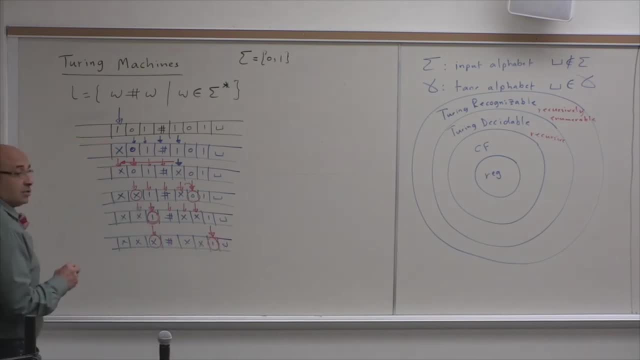 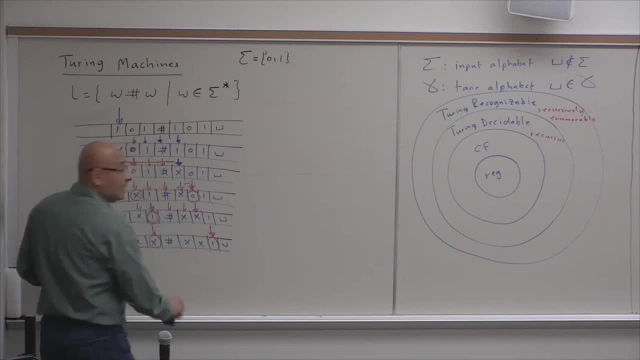 You can write, you can easily write a program that takes this as input and determines if you know the two strings on the on the two sides of this, this special symbol, if they are equal or not. So, basically, you write a program that does this. 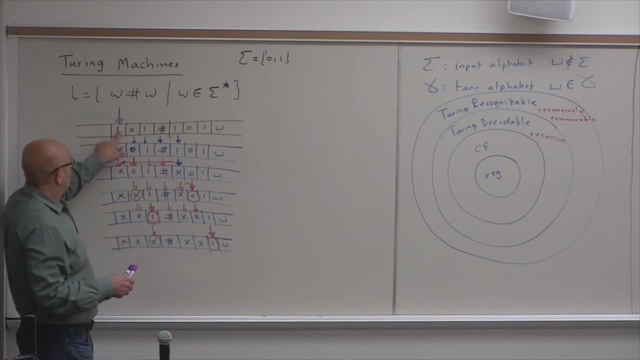 It's going to loop. It will check this and it will then. then it will compare it with the corresponding symbol to the right of the separator, And now it's going to mark this as an X. And we know that the, the string, belongs to the language. 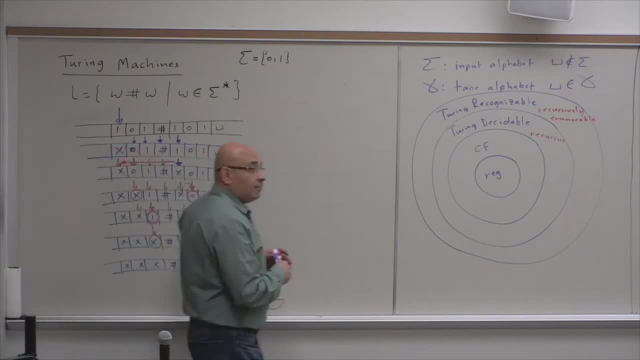 If what? If we are, you know, if we mark everything, if everything is marked, So you do a scan. If everything is marked, then the string belongs to the language. If it's not, if there is something unmarked, 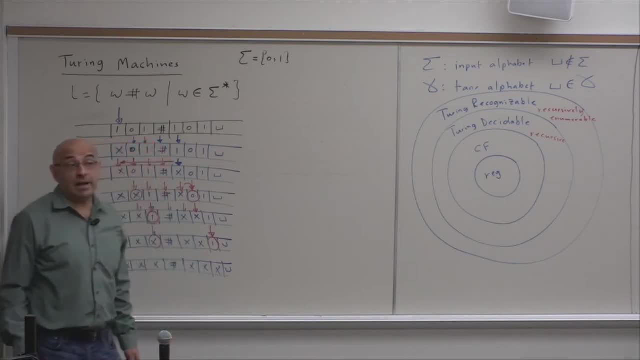 then the string does not belong to the, to the language, Or if any matching fails, like here. you know, if we had a say, if we had a zero here, If we had a zero here, then the first matching would fail. 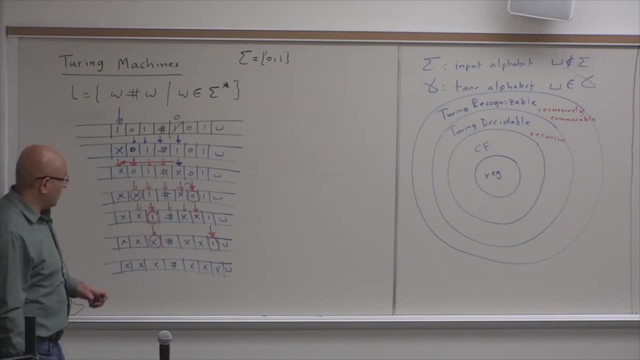 and then the two in one, And then the Turing machine would go to a reject state. So this is a problem that is Turing-decidable, It's a problem that can be decided by a Turing machine, Or in fact, it's a string that can be decided by. 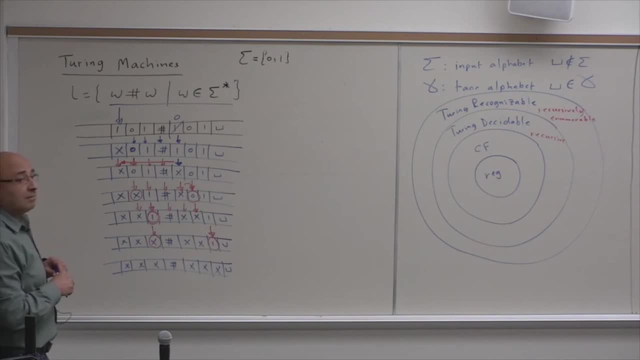 it's a language that can be decided by a Turing machine. So, yeah, so this looks like you know, this is you know this may look primitive. In fact, yeah, you can think of the Turing machine as a primitive model for a general-purpose computer. 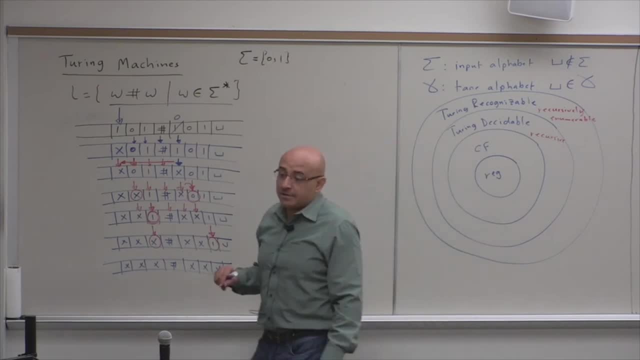 But it can do everything. You know it can do anything that a general-purpose computer can do. It may take more steps, But you can do with it anything that a general-purpose computer can do. Now let's look more closely into the transition function. 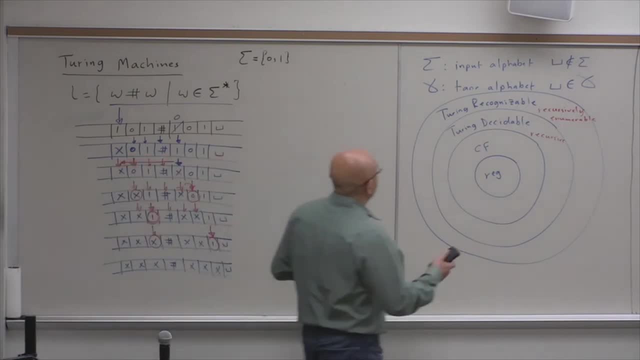 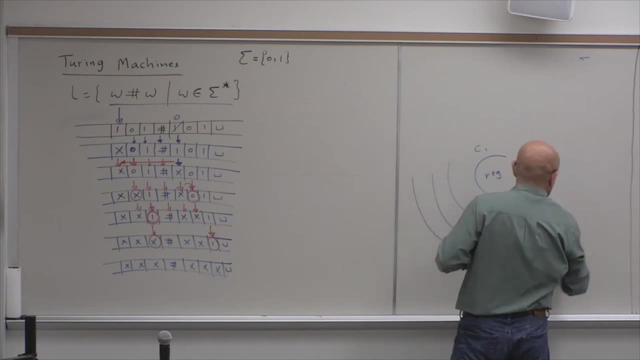 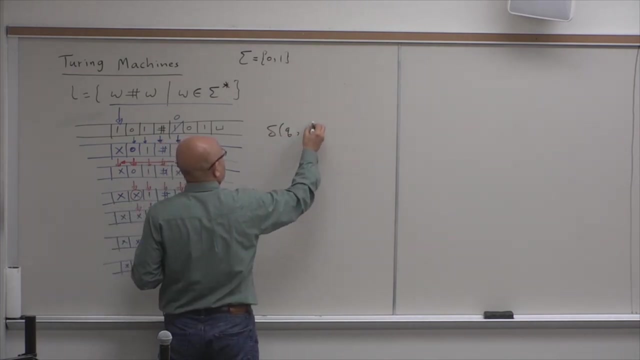 All right, So let's look at the transition function for a Turing machine. Oh, I need to do this. So the transition function, a transition function for a Turing machine, delta is going to take a state and a symbol and it's going to go. 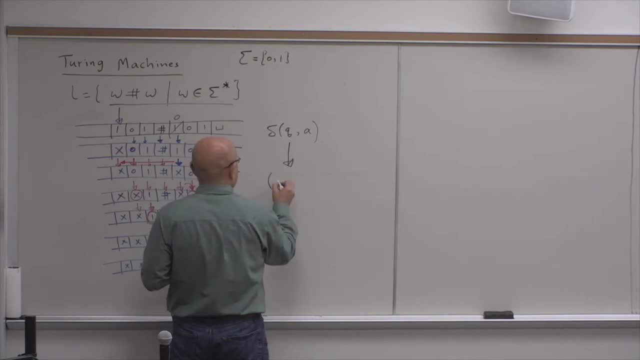 to a state, another state, another symbol and a left or right. Okay, So, for a small example, suppose that we have this Turing machine: This is A, B, B And we are in state Q0. And we have the tape here. 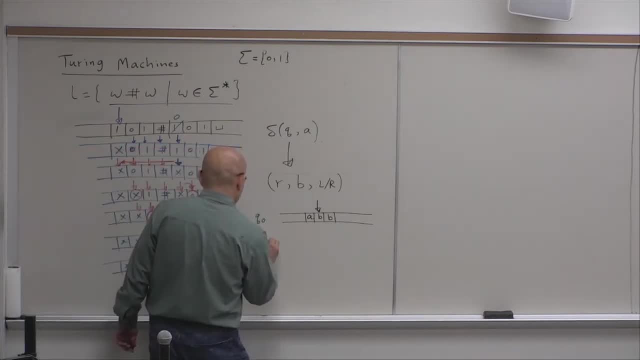 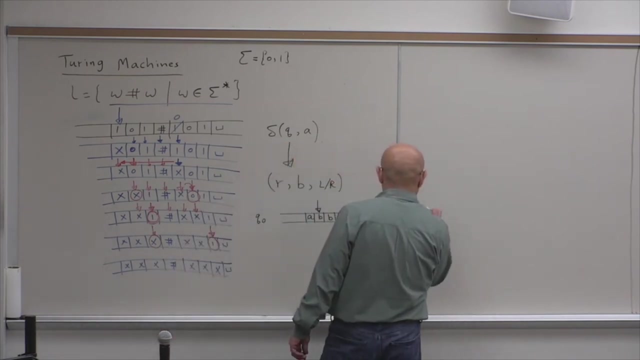 And we have: delta of Q0 and B equals, say, Q5 and C. or let's put it, let's not put it here, Let's put it here. Let's say: delta of Q0 and B equals Q5, C and right. 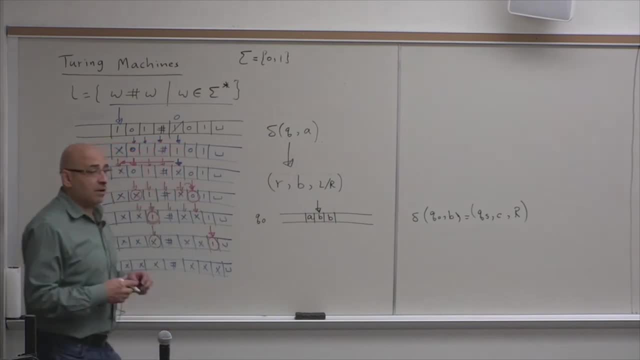 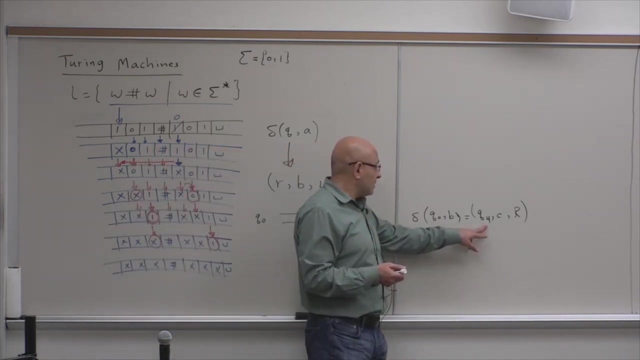 So the transition for a Turing machine should specify- and let's put it on so that we don't confuse it with an S, All right, So the transition for a Turing machine specifies the next state, current symbol in the input 2, and whether to go left or right. 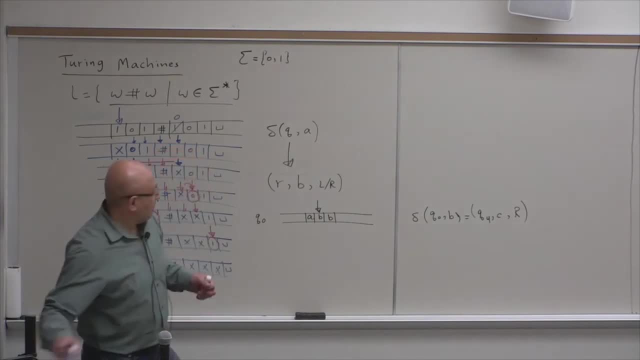 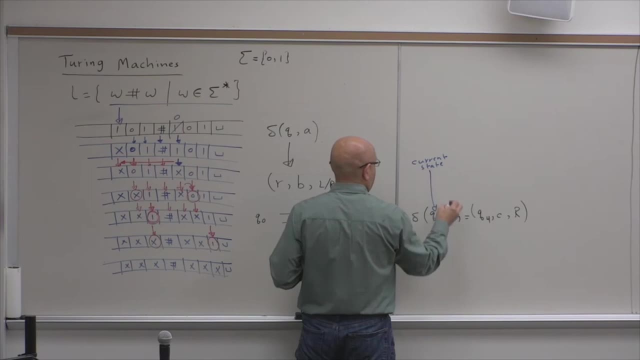 So this is. you know, this is what. This is the current state. This is the current symbol in the input, Current Symbol in the input. What's the definition of current symbol in the input? What the head is pointing at? 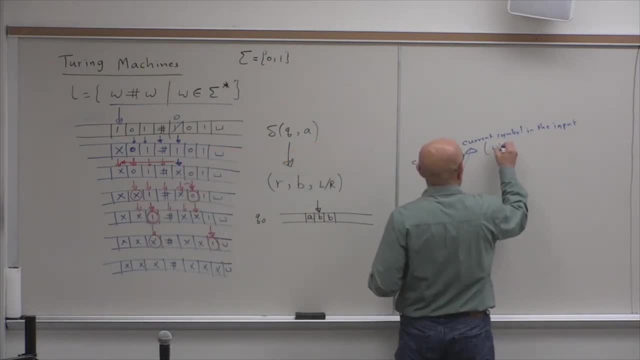 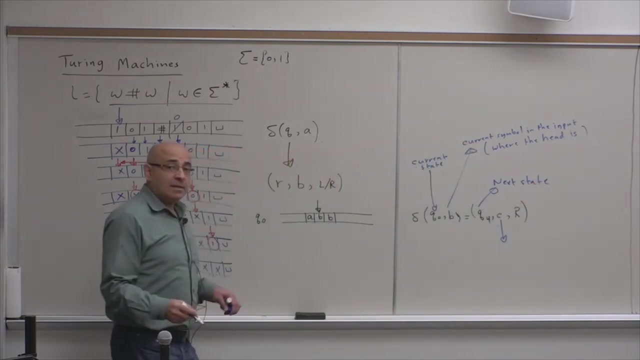 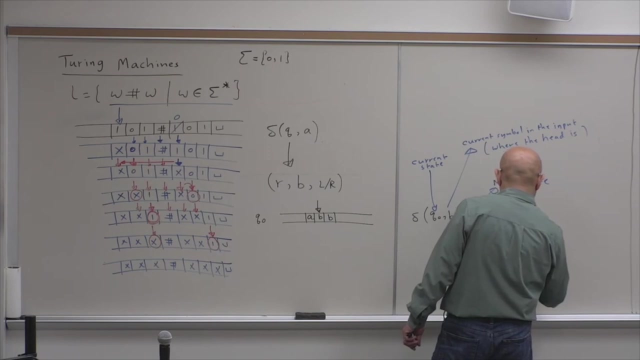 Where the head is. Where the head is And this Q4 is going to be next state. Okay, What's this C? This is what to replace the current symbol with. What to replace the current symbol with And what's the R? 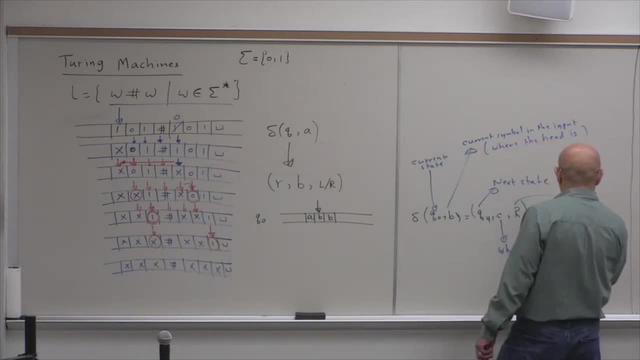 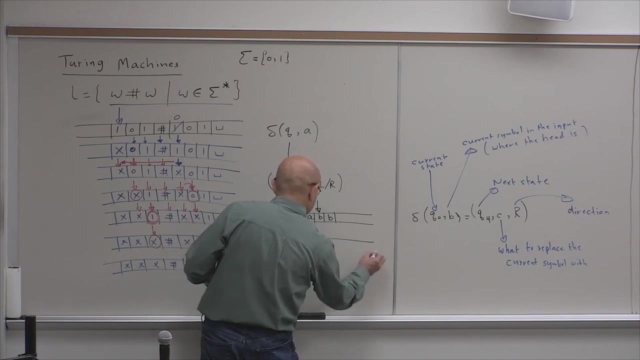 Go right Direction. Yeah, That's good Direction. Did they move him right after Q4? face the symbol: Yeah, We will show it right now exactly what will happen. So what will happen here? we will get this. So this B becomes AC. 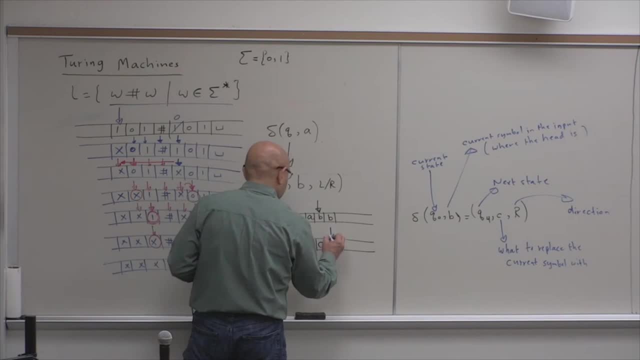 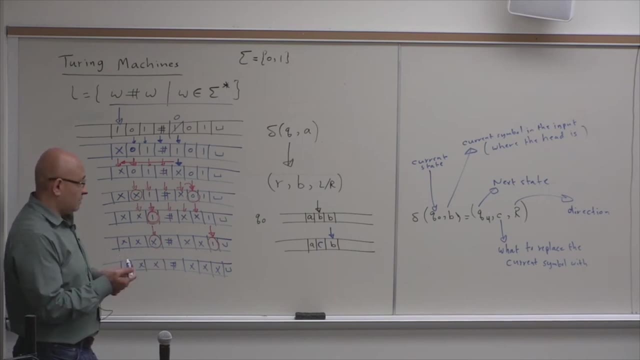 So we replace, Then we move to the right. So this shows us a single transition in a Turing machine And, as I said, you know, when we solve non-trivial problems, we will not be able to show this level of details for the Turing machine. 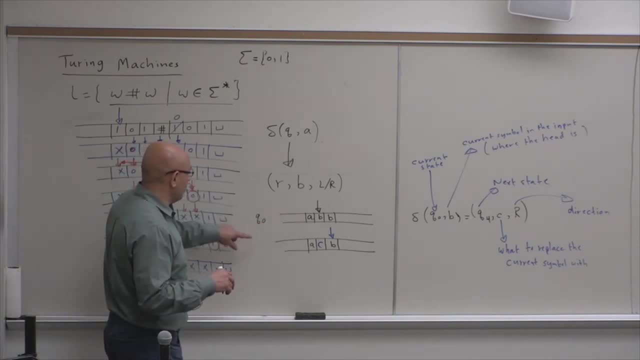 So if we are here and we apply this delta of Q0 and B is Q4, replace the B with a C. Okay, Okay, Replace a B with a C. So it basically says: change the state to Q4.. Your state becomes Q4. 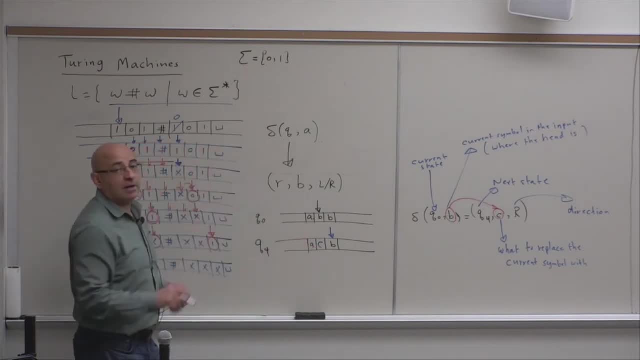 Your B becomes a C And move the head to the right. So if this had been an L, we would have put the head here Right. This thing had been an L instead of an R. Okay, We would have moved the head to the left. 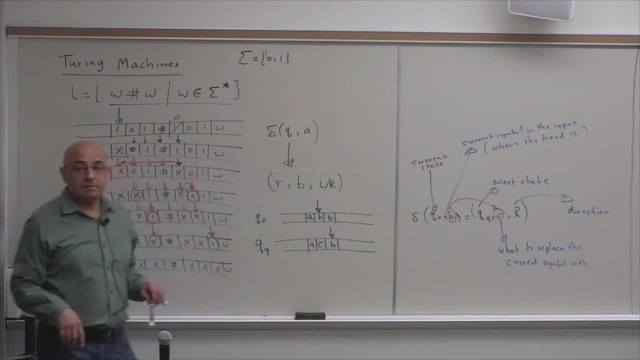 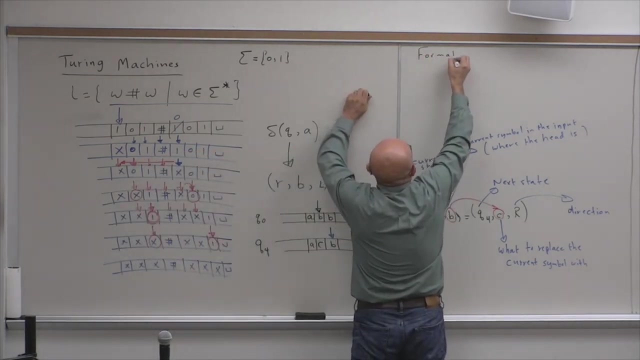 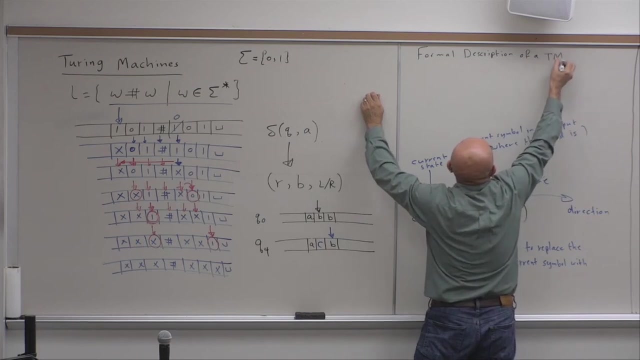 and we would have put the head here. Okay, So this is how it. you know it works. So let's now give the formal description of a Turing machine, Of a Turing machine. So a Turing machine is a machine that is a Turing machine. 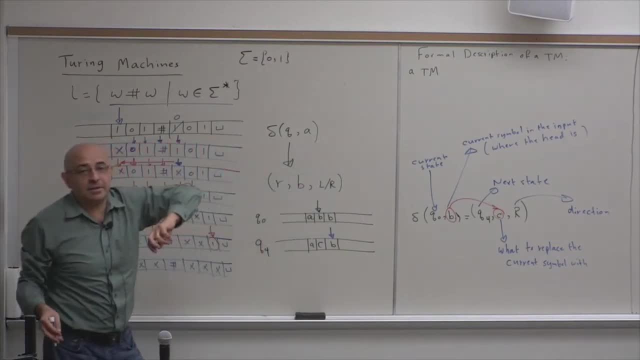 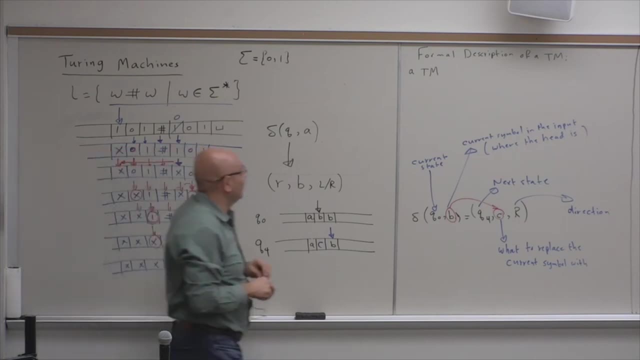 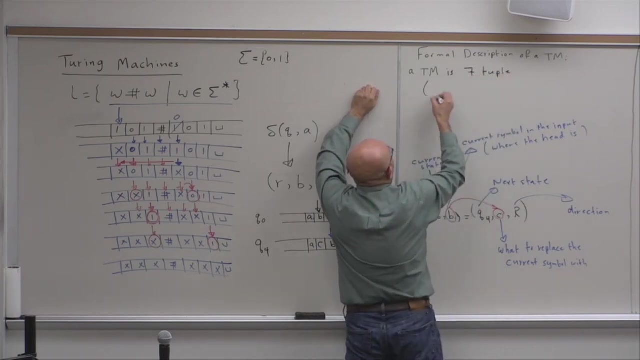 So the finite automaton was a 5-tuple, The push-down automaton was a 6-tuple And the Turing machine is a 7-tuple, Is a 7-tuple And it will have Q, sigma, gamma, delta, Q, sub S. 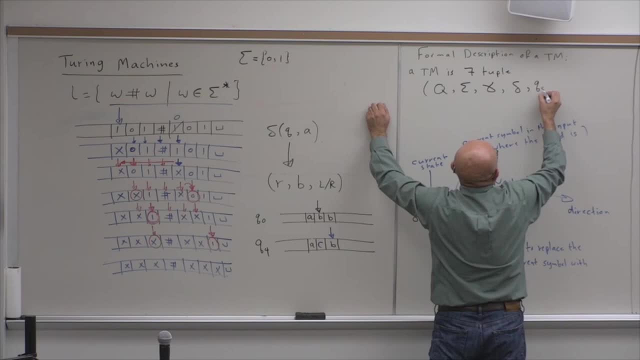 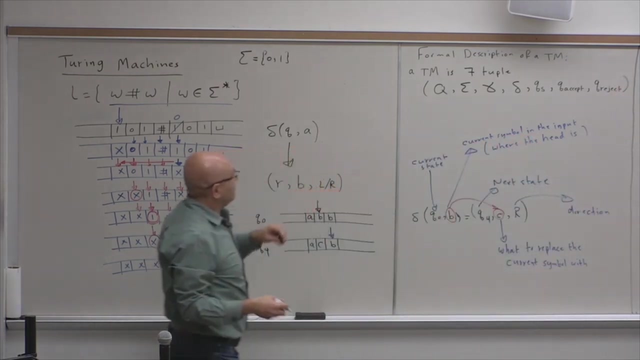 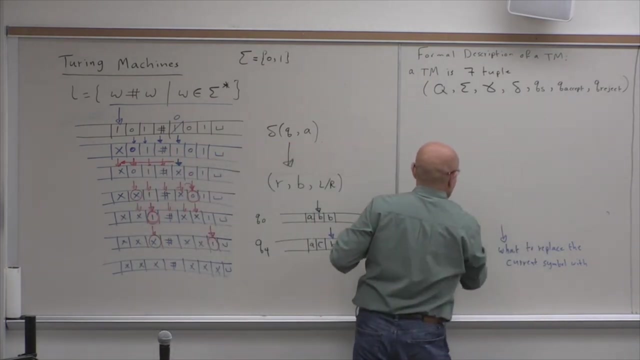 sigma gamma delta. Okay, Okay, So sigma gamma delta, Q sub S, Q accept and Q reject Now, so we are familiar with everything, in fact. So Q is a set of states. Sigma is what. Sigma is what. 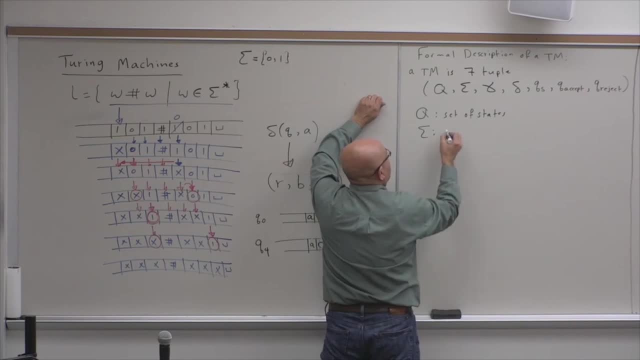 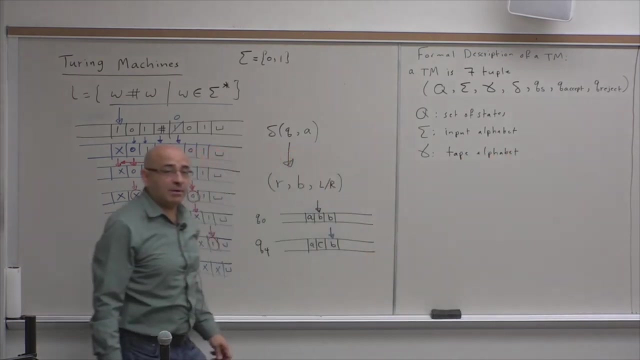 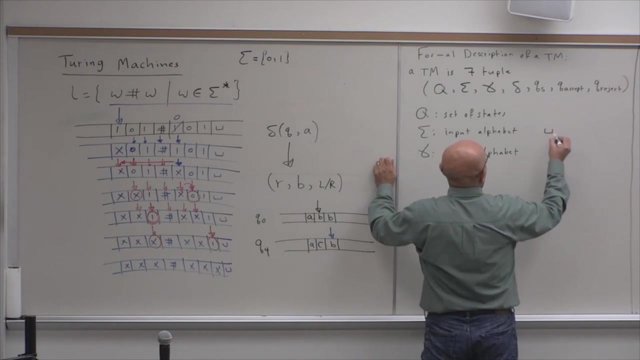 Sigma is what The input alphabet And gamma is the tape alphabet. So in push-down automaton we have the input alphabet and we have the stack alphabet And we have the end does not belong to sigma and it belongs to gamma And delta is the transition function. 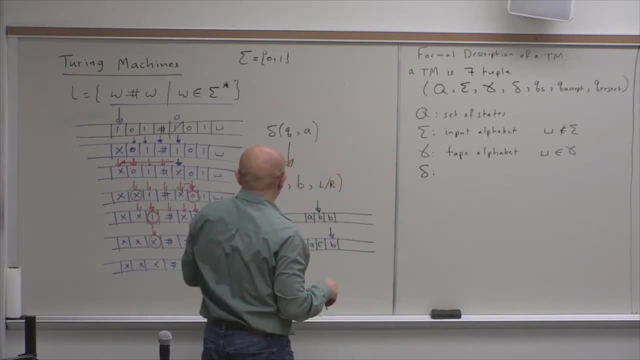 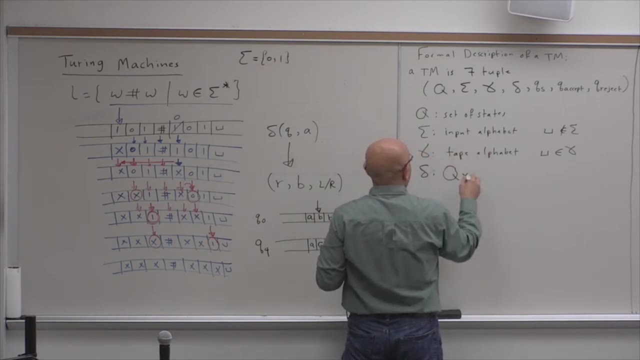 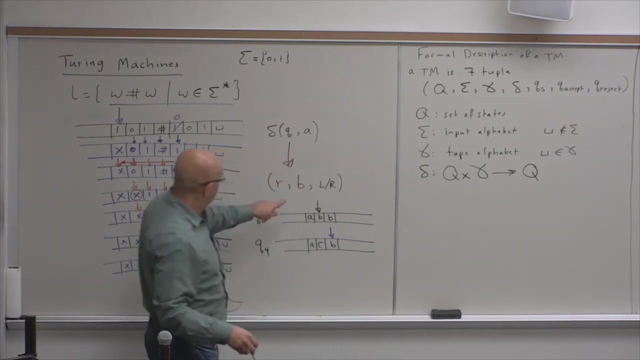 So the transition function in a Turing machine. it takes a state and a symbol in the tape alphabet and it gives you a state. It gives you a state. and what's this? A symbol in the gamma alphabet. It gives you a state. It gives you a state. 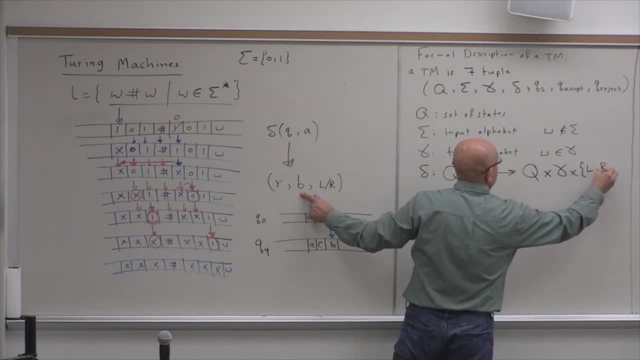 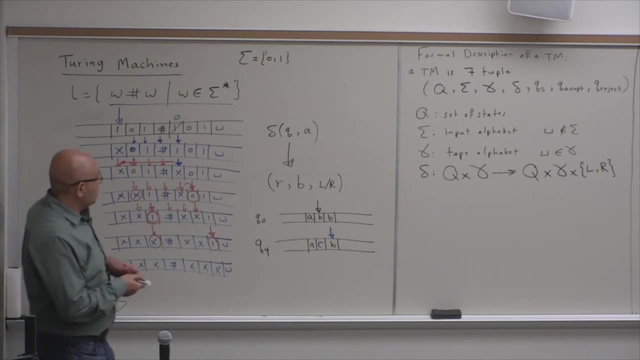 And a left or a right. So this is what the transition function in a Turing machine is. So it takes a state and a symbol from the tape alphabet, which is the bigger alphabet. The tape alphabet is the superset of the input alphabet, So it takes a state and a symbol. 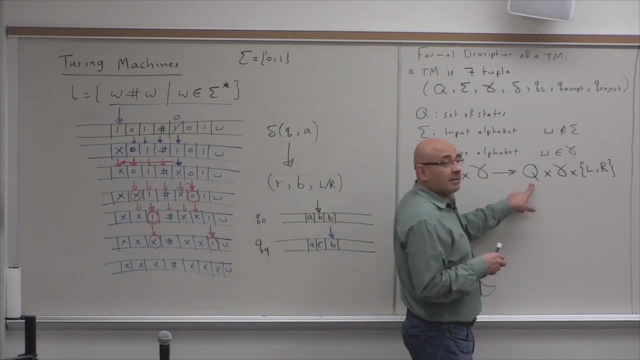 Okay, And it gives you a state symbol and it gives you a state. What's the next state? What should the symbol, the input symbol, be replaced with And go left or right? And QS is the start state. Q accept is the. 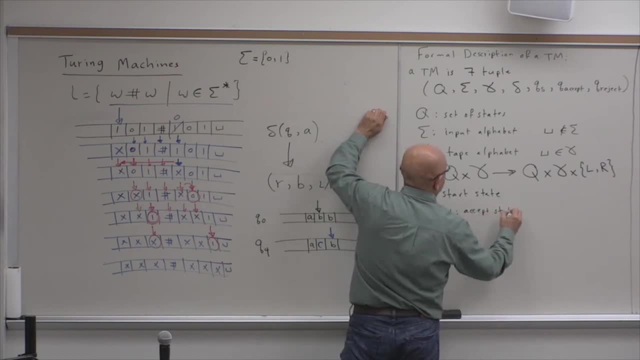 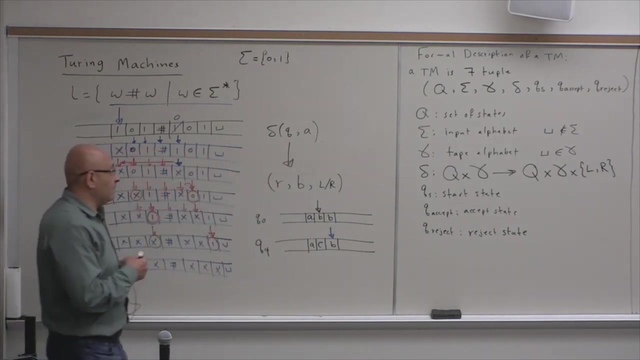 accept state And Q reject is the reject state. Now we have to have an explicit reject state. We have to have an explicit reject state because that finite automaton may not terminate within finite time For the. you know the finite for finite automaton: pushdown automaton. 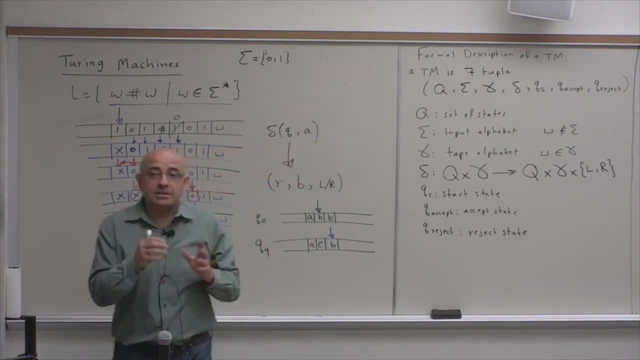 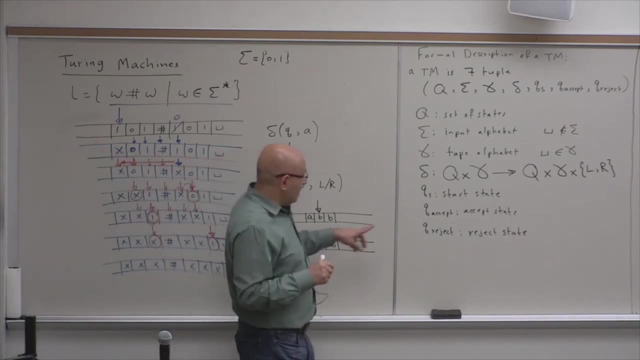 we know that we are done when we finish processing the string. We know that we are done When the string is completely processed. we know that we are done. But in the Turing machine we need a reject state because we need to know when to stop. because we can't, we can. 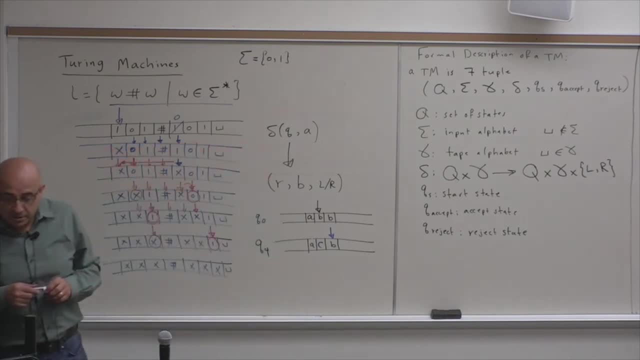 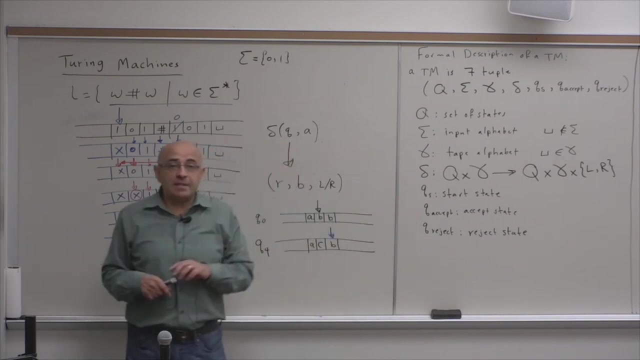 process the string multiple times. So you know, processing the string cannot be the determination condition in a Turing machine because you may process it multiple times. So you need an explicit reject state. Now, having one accept state does not. by having one accept state we do not lose generality because, as we have seen in NFAs, even if you 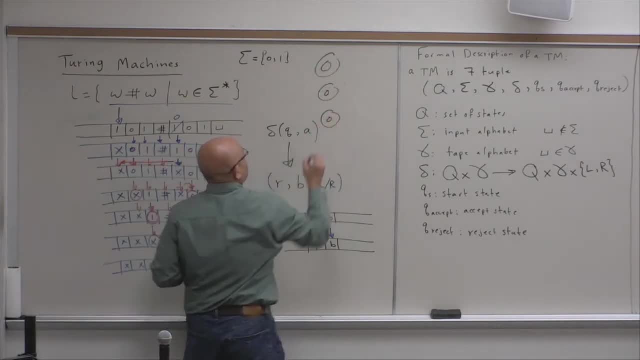 have multiple accept states, you can always have an epsilon transition, You know, you can unify them into one accept state And then these are no longer accept states. So if you give a, if you have an accept state, if you have an accept state, if you get an.